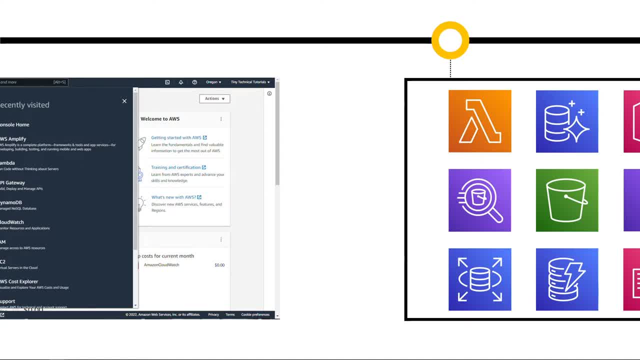 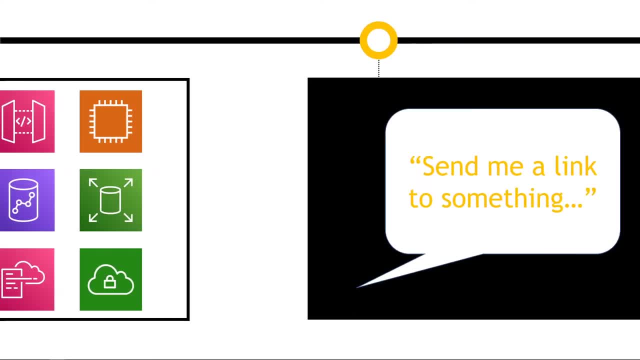 a new EC2 instance or create an S3 bucket and upload something to it And I felt like my learning was going along pretty well. But then one day I was telling some friends about AWS and how I was learning a new way to do development, And one of them said: send me. 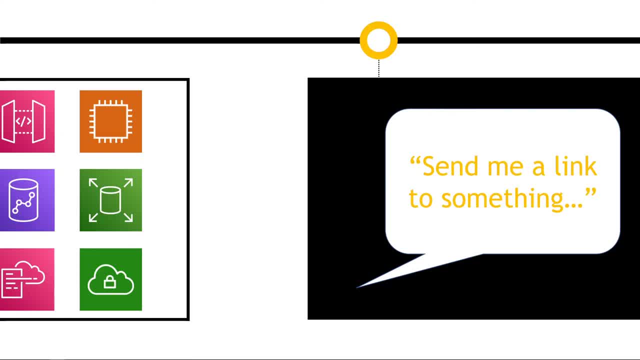 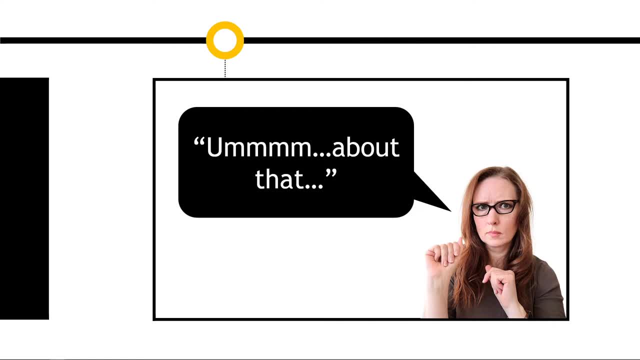 a link to something, because they wanted to check out my handiwork. Which made me stammer a little bit about that, Because it made me realize two things: One, I hadn't actually built anything that I could share with the outside world And two, and more importantly, I didn't actually know. 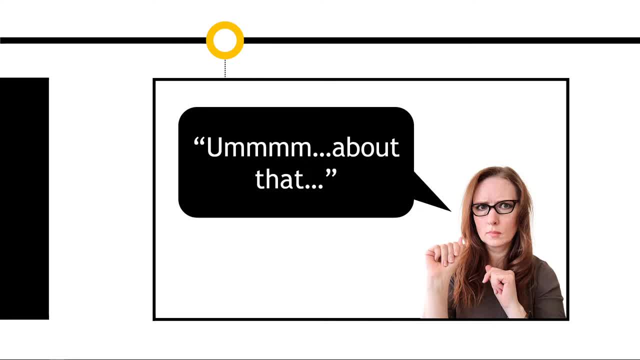 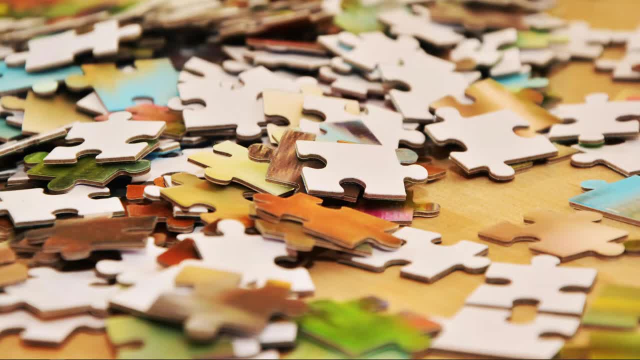 how to build something, because I wasn't able to put all the services together into an actual application. I knew what the puzzle pieces were, In other words, the different AWS services I had been learning about, but I wasn't able to put them together into an actual, usable thing. And if 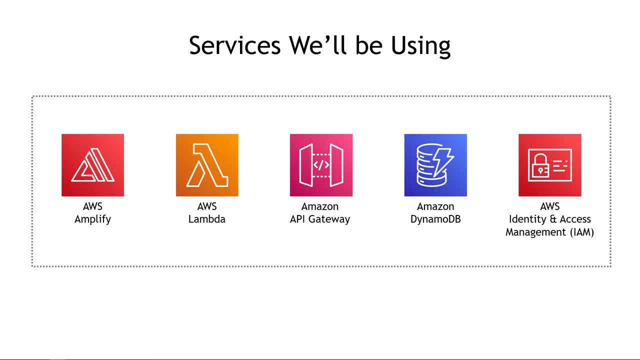 you're feeling the same way, you've come to the right place. In this video, we'll be using five AWS services shown here to build an end-to-end web application from scratch, And, yes, you can even share it with your friends when you're done. if you'd like, Let me show you the working version. 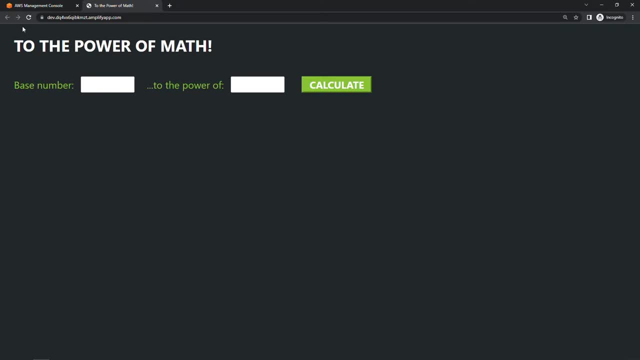 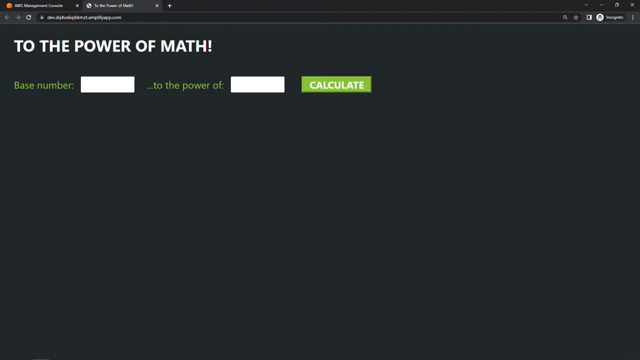 much larger real-world application. This just takes in two different numbers. So we have a base number, let's say two- and then an exponent. We'll go with five and it's going to return the result, the base, to the power of the exponent. If we click on calculate, the result is 32.. You'll see that we 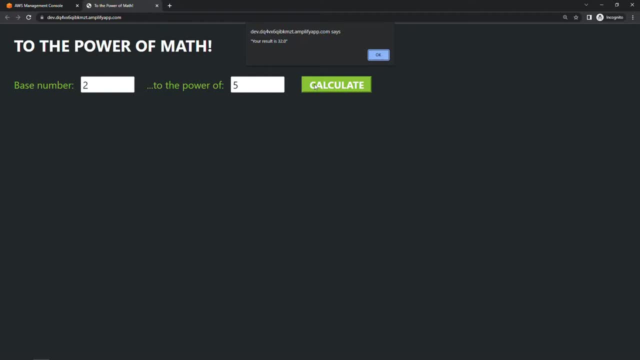 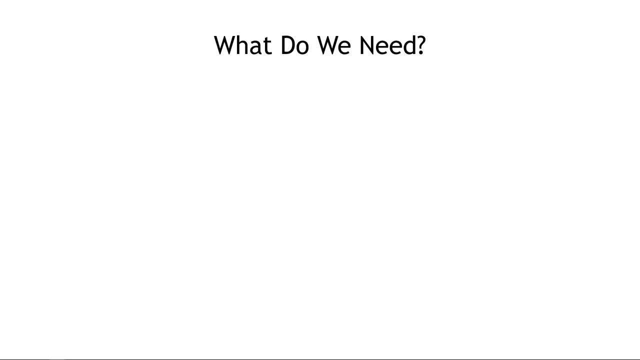 get that in the pop-up. It's also being saved to a DynamoDB table on the back end if you wanted to do something with it down the line. All right, now that you've seen that very exciting application that we're working towards, let's walk through how we got there. What do we need to do to make this happen? Well, 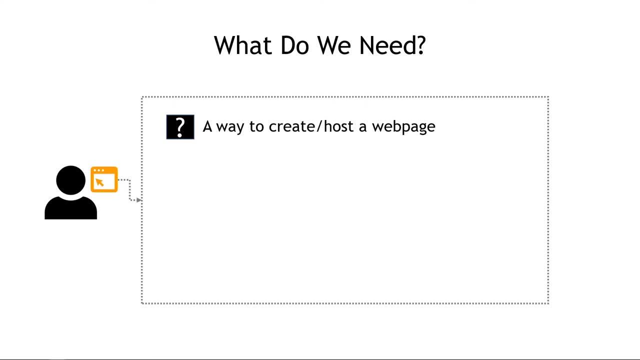 first, we need some way to create and host a web page. This is what your users will navigate to in their browser. We need a way to invoke the math functionality. We need a way to actually do that math, to do the calculation that we saw, Somewhere to store the result. 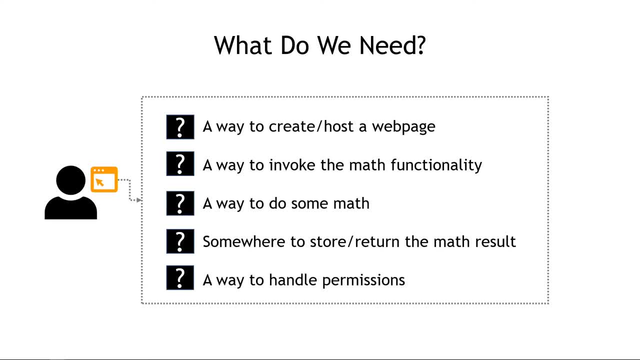 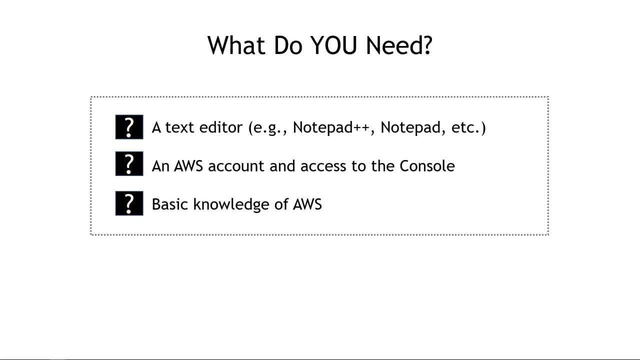 and we also need to return the result to the user, And then sort of a given is that we need to handle permissions along the way as well. And before I get ahead of myself, if you're following along with me, you are going to need a text editor, something like a Notepad++ or Notepad. 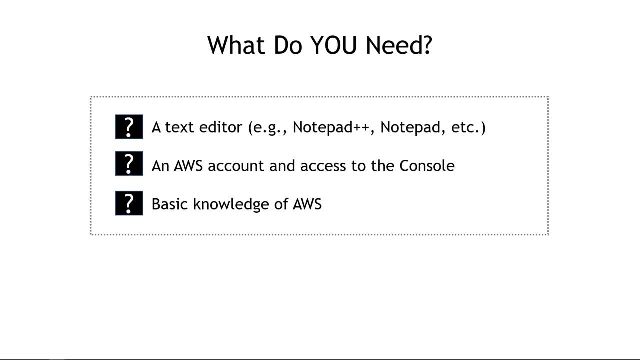 whatever your favorite editor is, You'll need an AWS account and access to the console Link above and below on how to set that up if you don't have one already, And then a basic knowledge of AWS. This video isn't meant to be a deep dive into any of those five different services I mentioned. 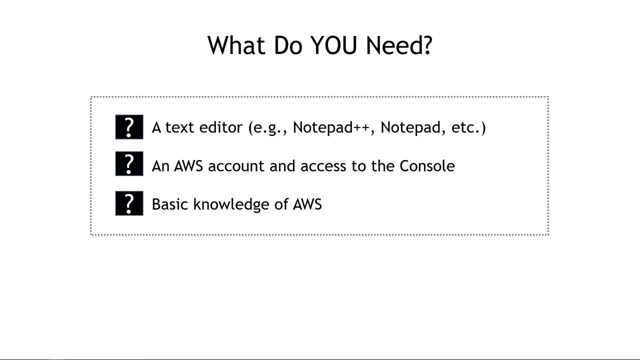 but it's really to help you tie them all together into a working environment, So let's go ahead and get started. So if you have some basic understanding already, that will be helpful. If you don't, though, you should still be able to follow along as I'm building out the app. 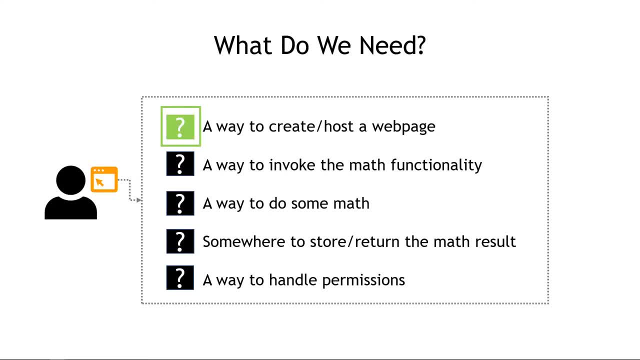 So back to what we need to do for this application. We need a way to create and host a web page. How would you implement that in the land of AWS? As with most things in AWS, there's actually several ways you could do this. The one we're going to choose just because it's super easy. 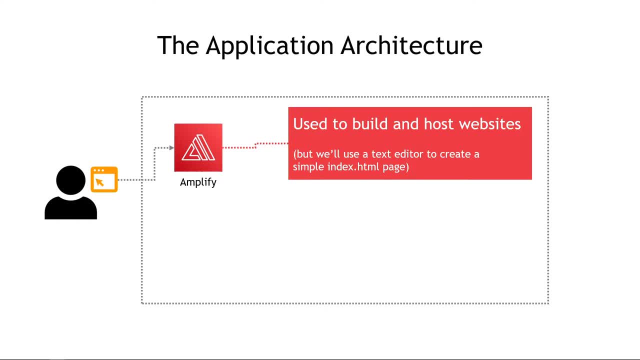 is called Amplify. With Amplify, you can build and host websites and it's a great service, particularly if you're a front-end developer. If you're a front-end developer, you can build and host websites and it's a great service, particularly if you're a front-end developer. 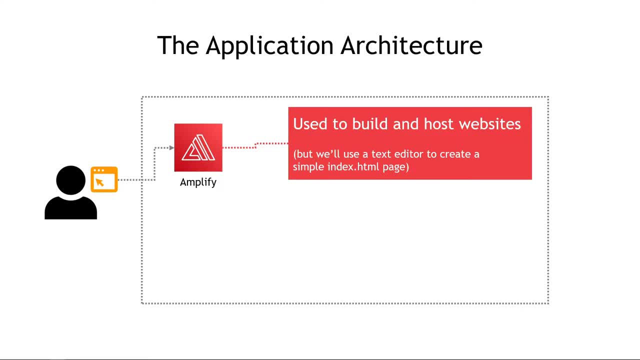 But for our purposes, since our page will be so simple, I'm actually just going to go create an HTML page in my text editor on my local machine, and then we're only going to use Amplify to deploy and host that web page. So let's go do that now. So here on my local machine, I'm just going to. 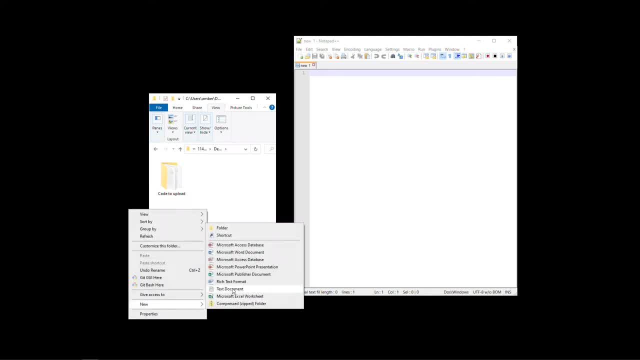 create a new. I'll start with a text file and we'll call this indexhtml. You can get rid of the txt. Yes, we want to change this. We want an HTML file. We're going to call this indexhtml. 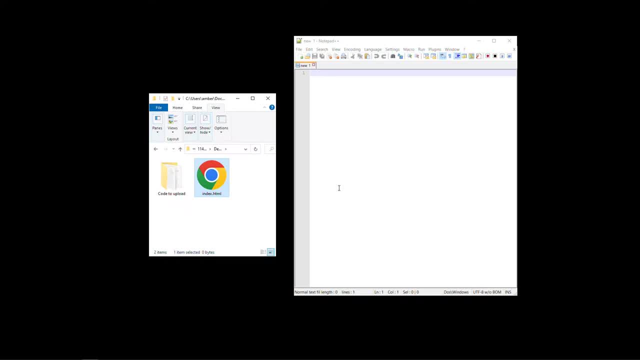 Or if you have a preferred way to create a new HTML file, you can go ahead and do that. But let's open this one up. I'm going to use Notepad++ over here and I'll just paste in some really simple code here where we're basically just going to display to the power of math the name of our 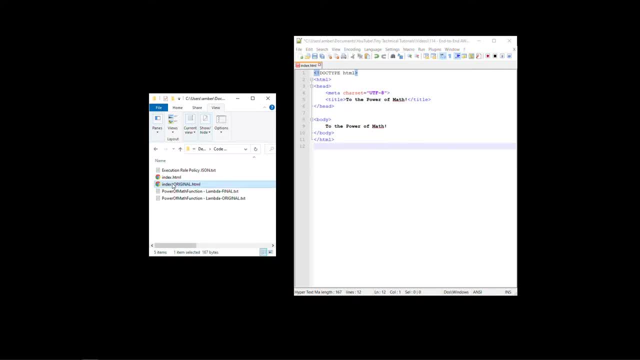 application. Now all of this code. incidentally, I'm going to upload and link it in the description below, so don't feel like you have to type all of this out. This one will be called index-original. We are going to update this later to be a little bit more robust, but this is the one. 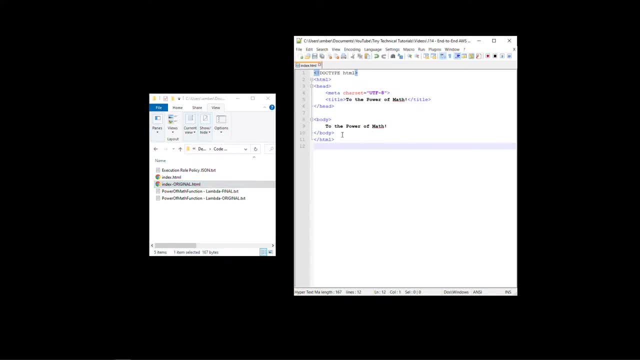 you want, if you're looking at the description. So let's save the file and then what we need to do is zip it up. So zip up just the indexhtml file. In my case that will be sent to compressed folder, or if you have some other way to zip up your files, do that. So you should have one zip file called. 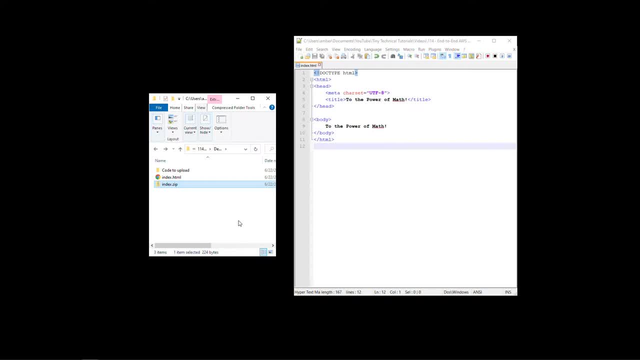 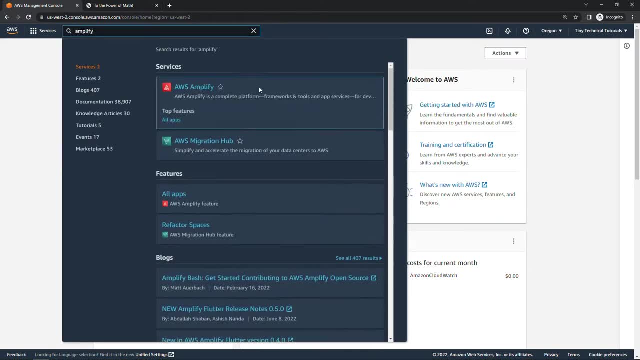 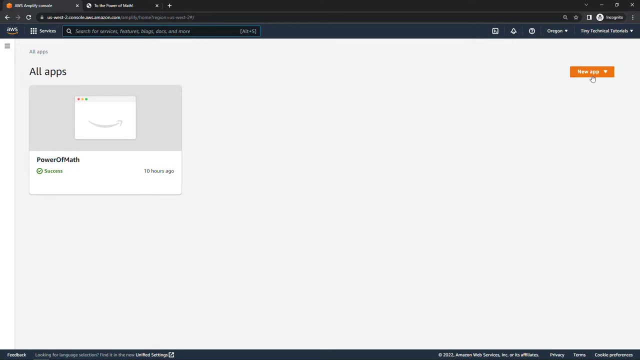 index, And now we're going to use Amplify to deploy that Here on the AWS console. navigate to Amplify. Now I do have one app here already. This is the completed app that we saw a minute ago, So I'll create a new app, and here we just want to host the web app. We don't have a get provider. 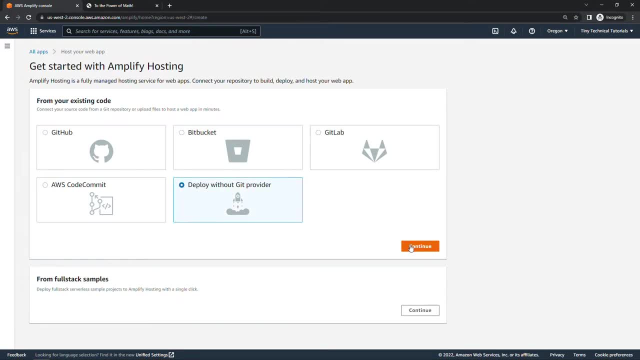 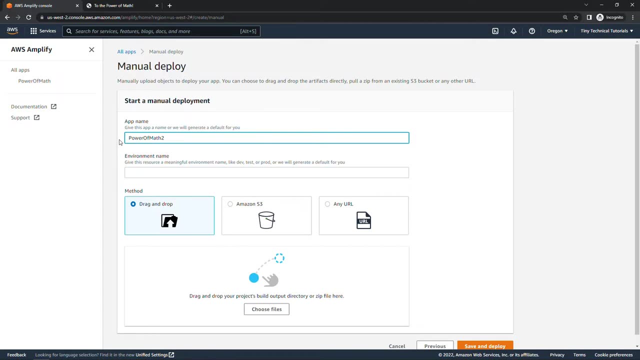 so you can select this option right here and continue. Give the app a name. I'm going to call mine Power of Math 2,, since I already have an original one: The environment name. I'm going to use dev and we want to drag and drop. So here's where you grab that zip file that we created a. 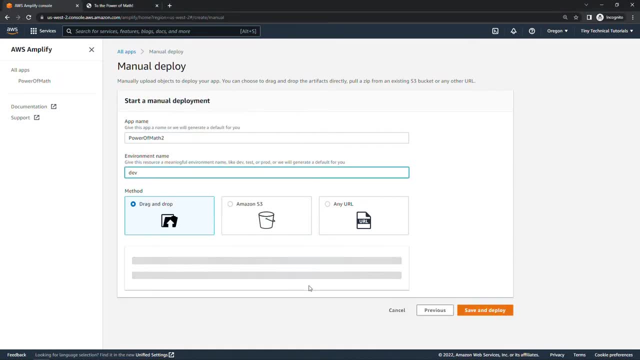 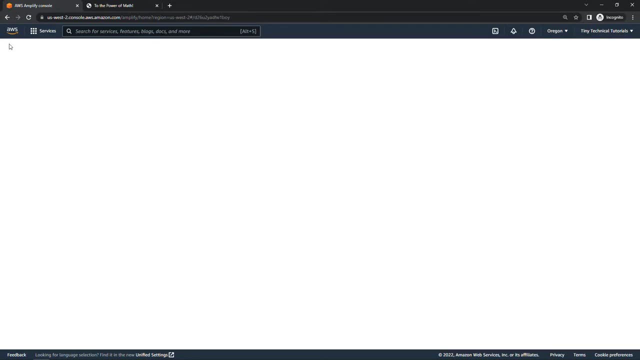 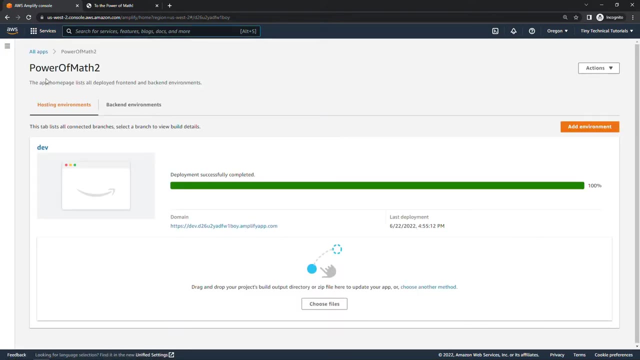 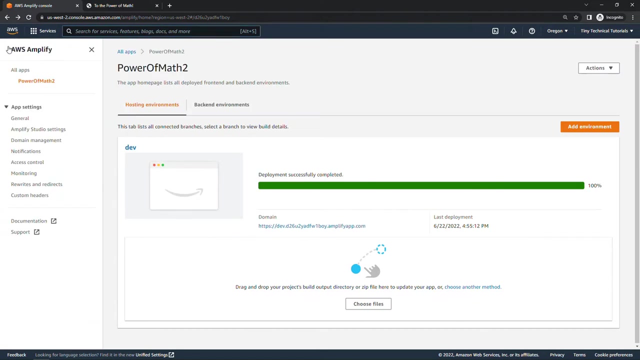 while ago. Just drag that over, save and deploy, and I don't know if this is a small bug, but you might need to refresh. Sometimes my screen just goes white there. but you'll see. deployment is successful And here is your link. You can also get to this anytime by coming over to domain. 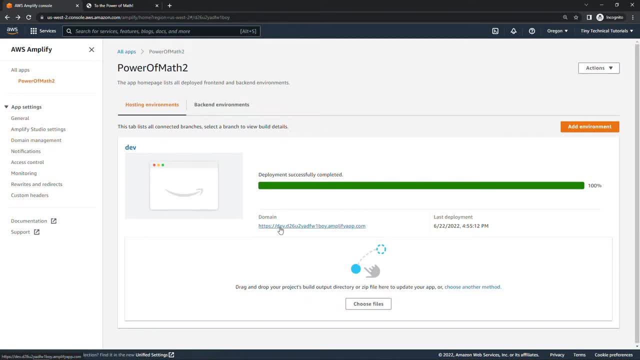 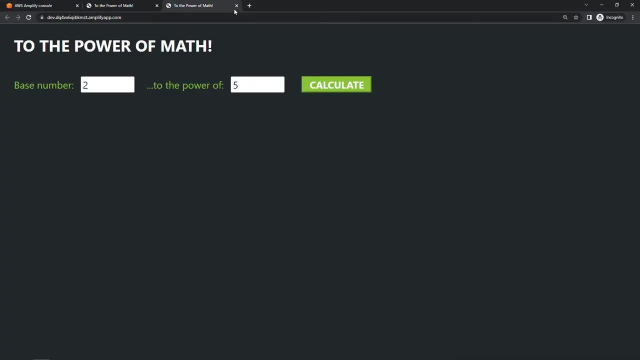 management and you can access those links as well. open this in a new tab. I have the original one open here too. Let me just close that so I don't get confused. This is the one that we just deployed our simple indexhtml page to the power. 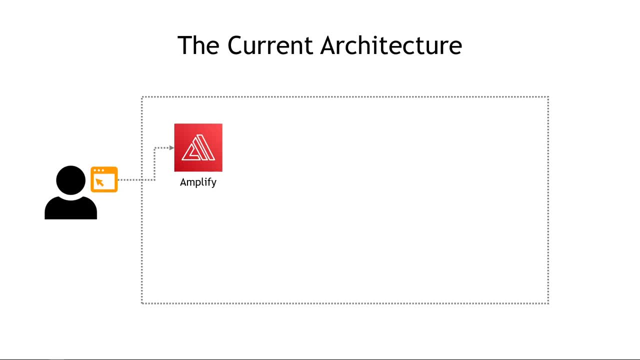 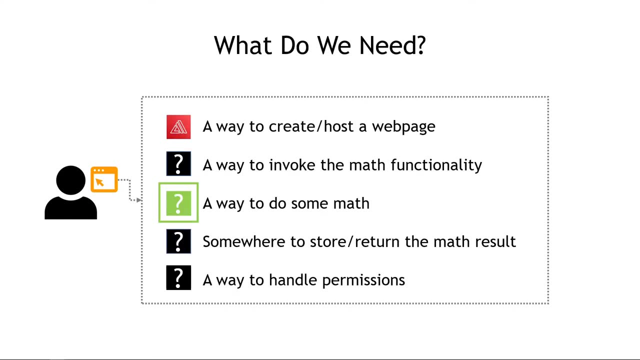 of math, Yay, All right. so here's what we have so far: Super simple, but we now have a live web page that users can navigate to Back to our list of things to do. I'm actually going to skip around. 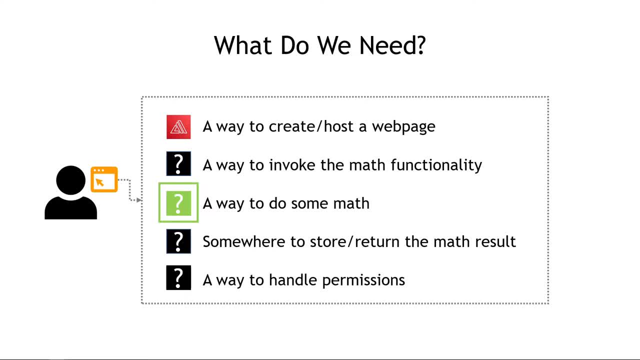 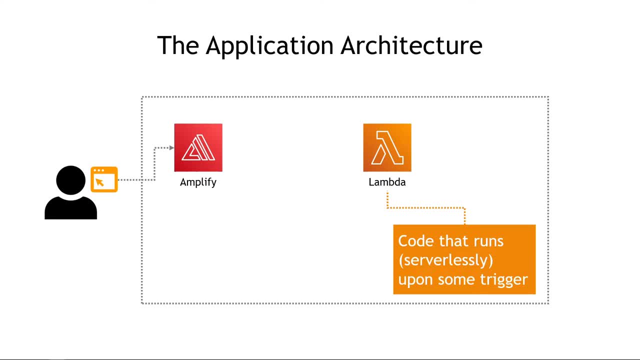 a little bit here to this item in green and we're going to work on a way to do some math. To do this, we're going to use a lambda function. As you might know, a lambda function is just a bit of code that runs in response to some trigger, For example, when you upload a picture to an S3 bucket. 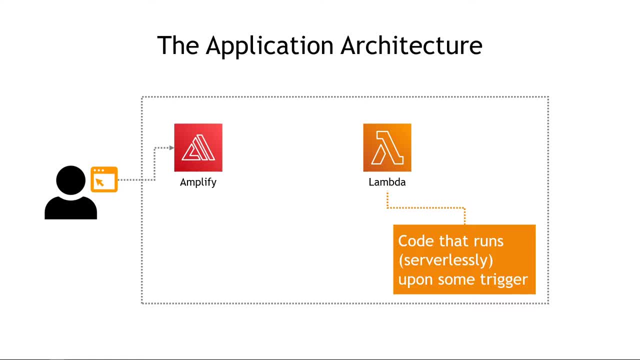 that could trigger a lambda function to go process the picture into a thumbnail or something like that. It's just code or functions really sitting out there that get run when you need them, And these are serverless, meaning that you don't have to set up and manage servers to run the code. 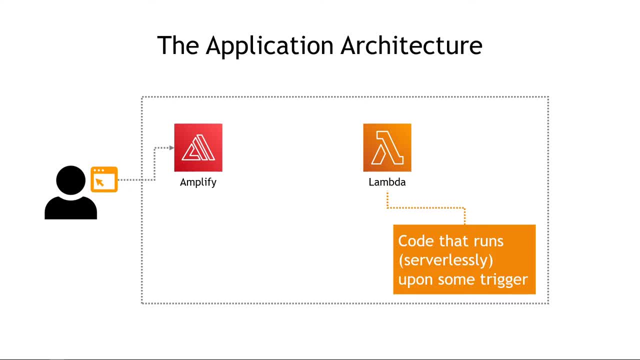 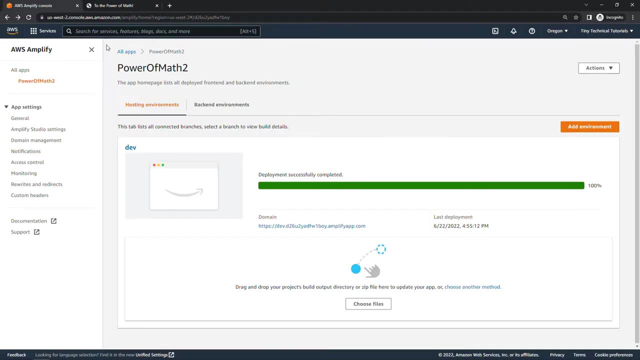 It just happens automatically behind the scenes for you. So we'll write some Python code and use it to run the code. So let's go ahead and run the code. We're going to use the Python math library to do the calculations that we need Back here on the 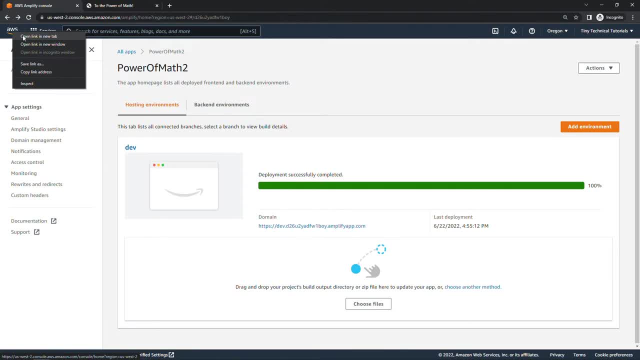 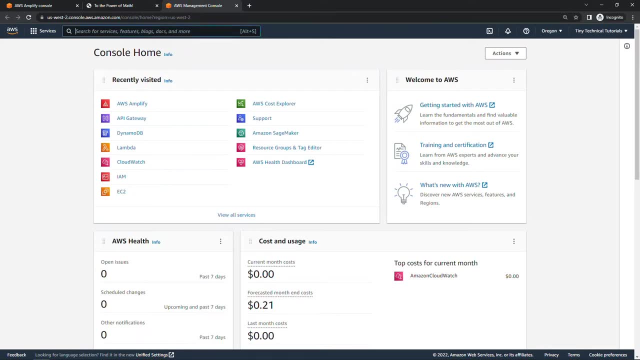 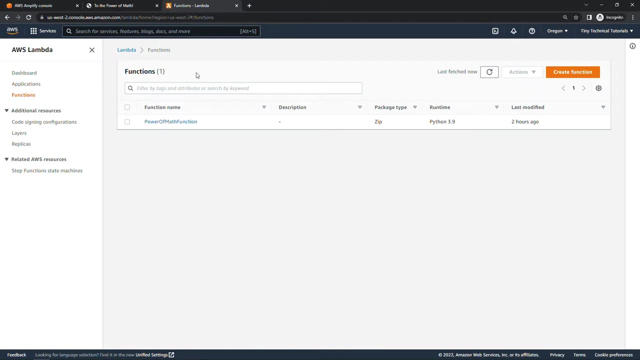 console, go ahead and open up a new tab here, just so we can keep Amplify handy. And this time we're going to navigate to lambda. Once again, I have the function that I was using for my original application. I'll create a new one and we're going to author this from scratch. That should. 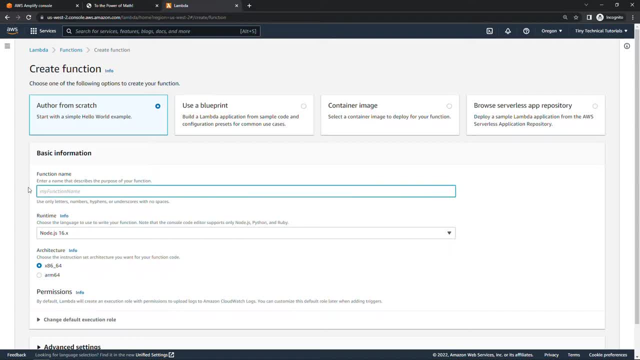 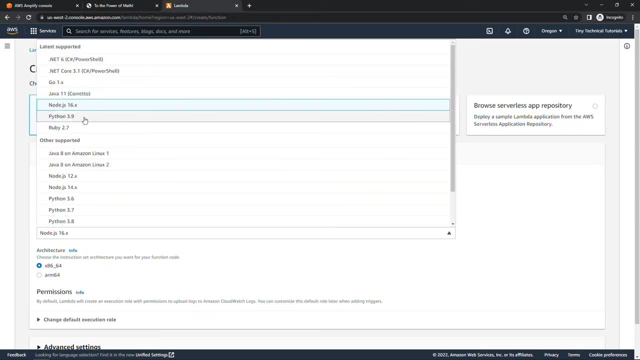 be your default already. And then for function name, I'm going to do power of math, function two in my case. For runtime, let's go with the latest version of Python 3.9.. You can leave everything else the same and create function down here on. 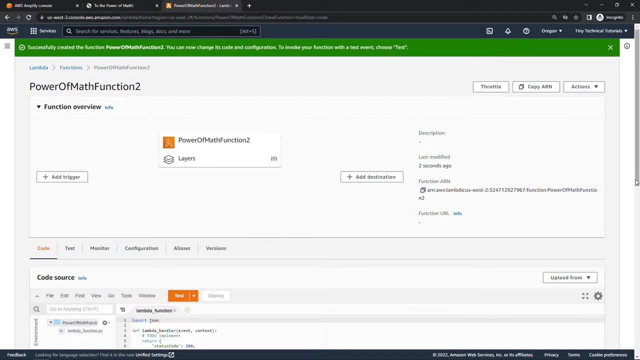 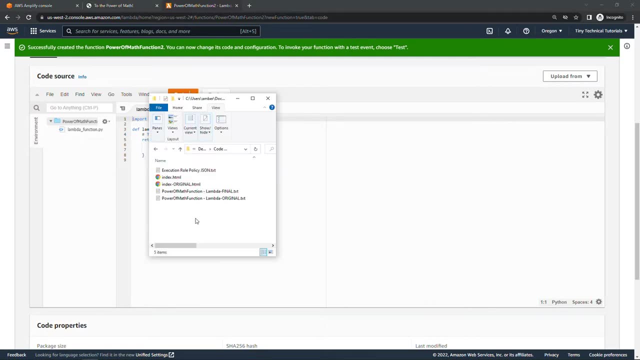 the lower right. All right, this code down here we're going to need to update. Let me go grab that from my desktop. Once again, if you're getting the code from the link in the description, you'll want the one that says lambda original. We are going to update this later, so I wanted to keep. 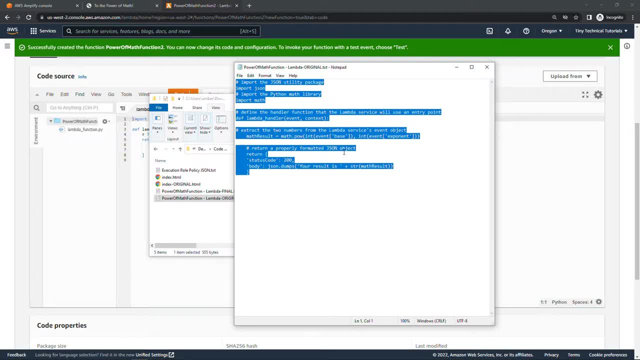 them separate. But let me just go ahead and do that, And then we're going to do power of math, function two in my case. So let me just grab this and then I'll walk you through it real quickly. You can replace everything here. So pretty simple code. We're just importing the. 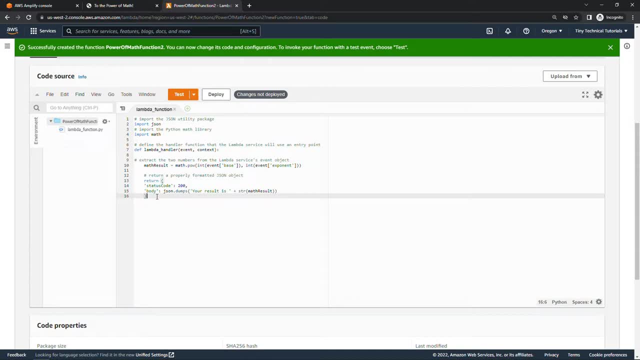 JSON utility package and the Python math library so we can do our calculation. Then you've got your lambda handler. This is common to all lambda functions And here's where we do most of the work. This is where we're getting our math result. So remember that our user is going to be passing. 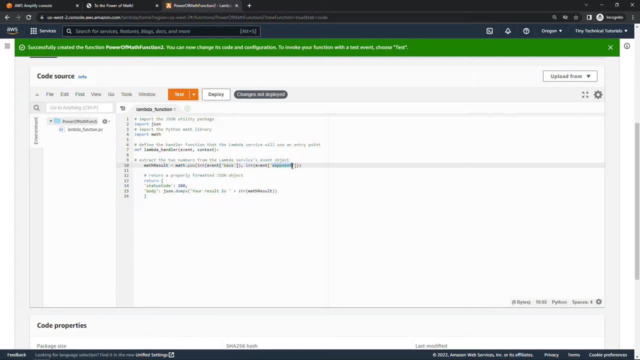 in two numbers: the base number and then the exponent. We're grabbing those out of the event object that we'll get and then plugging them into this math dot pow for power which is going to give us the result, And then we'll return that result down here in the JSON object. All right, 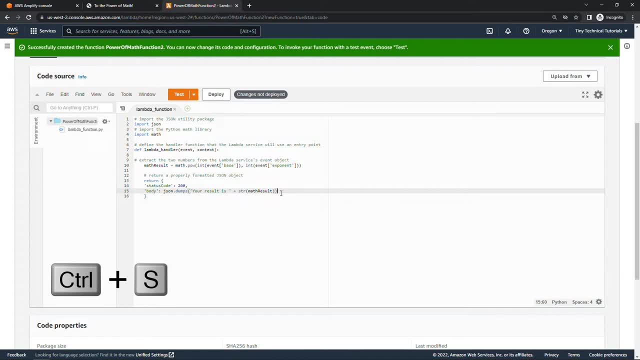 make sure you save this code. you can just do Ctrl S And then, very importantly, you also need to deploy it. So this button right here, And now let's test to make sure this functions as we expect. So click the little drop down arrow right here to the right of test And let's go set up. 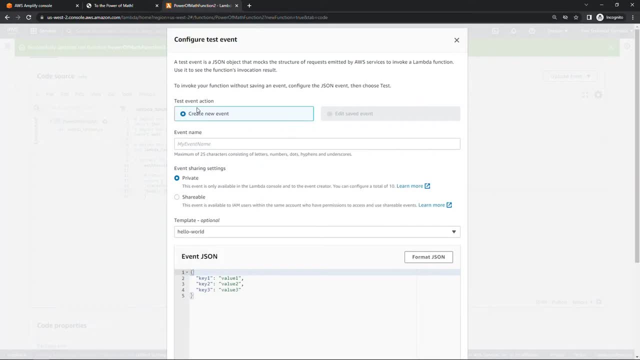 a test event. This basically lets us pass in some test data to make sure that the function is working. So create a new event. event name: power of math test event. In my case, I'm going to do two. you can leave this private And then down here it's giving you some starter code. We only 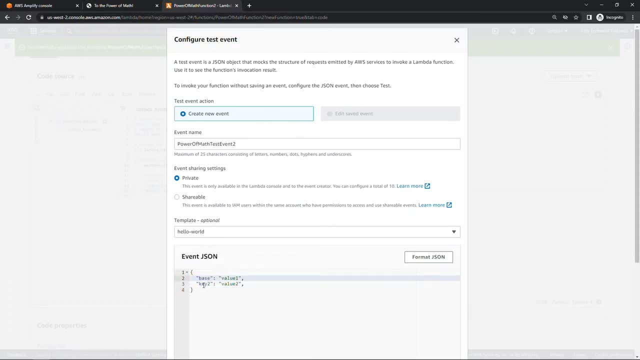 have two values to pass in. one of them is going to be base and one is going to be exponent, And you can choose whatever values you want here. I'm going to go ahead and do that And I'm going to do two to the power of three, which should give us eight, So we can test that that's working scroll. 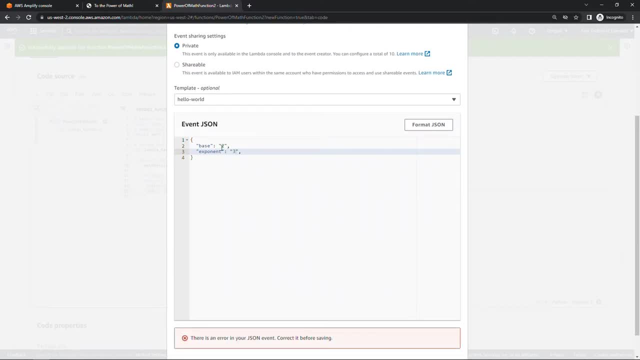 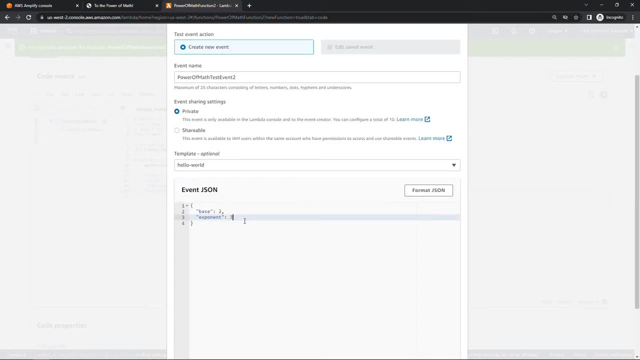 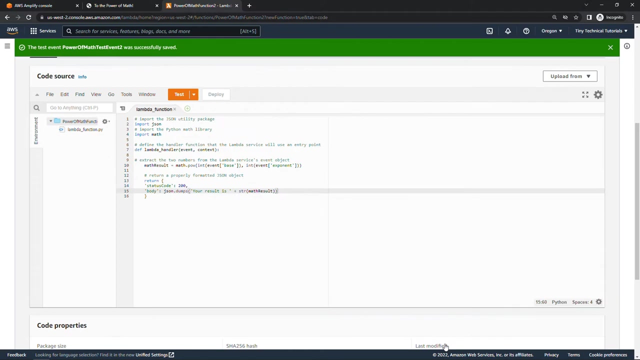 down and then save. My bad, we don't need quotes around those numbers. If you are using strings, you would, okay, make sure you get rid of that last comma there as well, And then scroll down and save. So that was just configuring the test event. Now we need to actually run the test, which you can do. 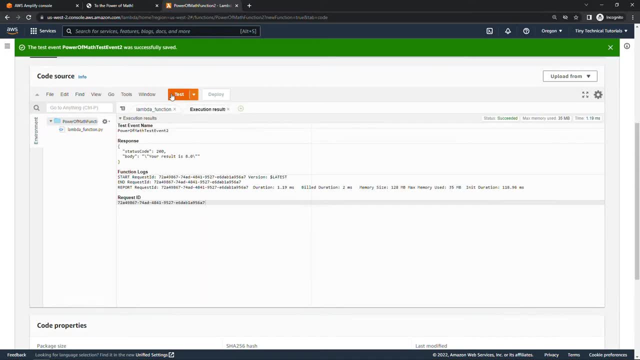 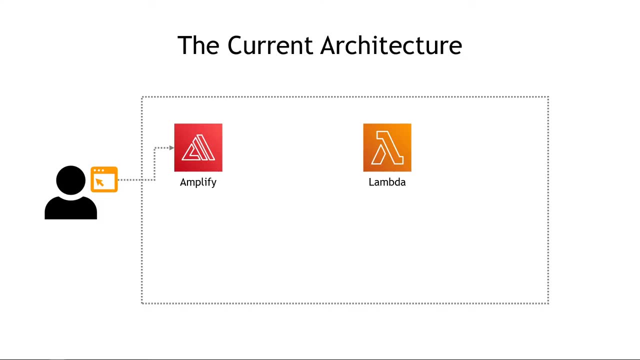 right here by the orange test button, And then we're going to go ahead and run the test And we get a status code of 200. And the result is eight. Perfect, So our lambda function is working All right. this is what we have so far, just the simple HTML page hosted in Amplify and a lambda. 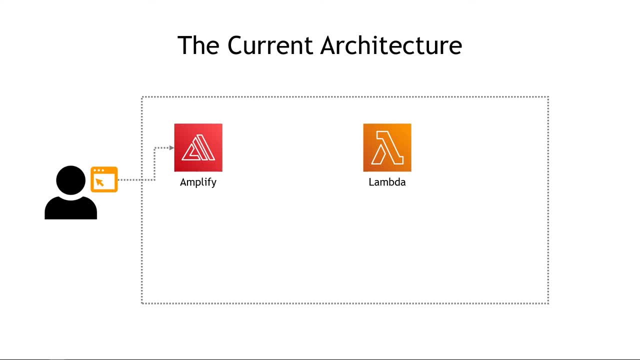 function to do some basic math. What's next? Well, next you need to go hit that like button If you're enjoying the video. I'd really appreciate it. It does help the contents spread to more people And also think about subscribing to the channel. Thank you so much. All right back to work. Next, we need a way to integrate the code. So we're going to go ahead and do that, And we're going to go ahead and do that, And we're going to go ahead and do that, And we're going to go ahead. 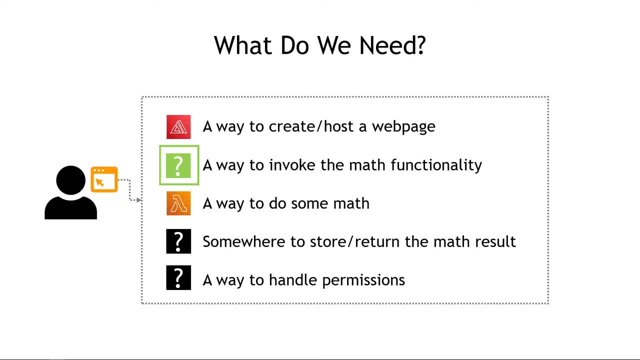 invoke that math functionality or basically invoke that lambda function. So our users obviously aren't going to go into the AWS console like we just did and run it. So we need a public endpoint or URL that can be called to trigger that function to run, And for that we're going to use 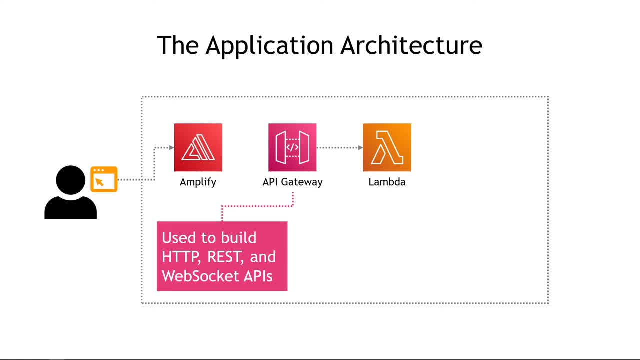 API gateway. This is a core service in AWS that you can use to build your own APIs, application and programming interfaces, whether those are HTTP, REST or WebSocket APIs- And it's really the perfect way to invoke a lambda function. So let's go ahead and do that, And we're going to go ahead. 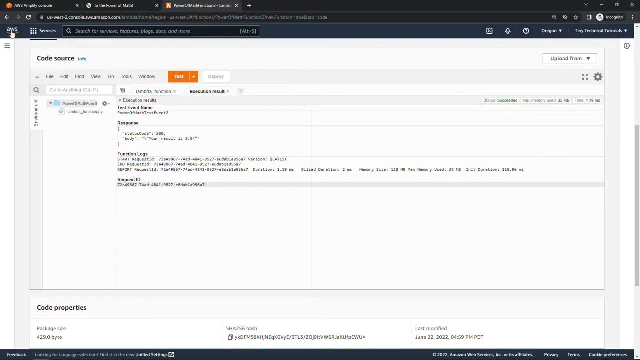 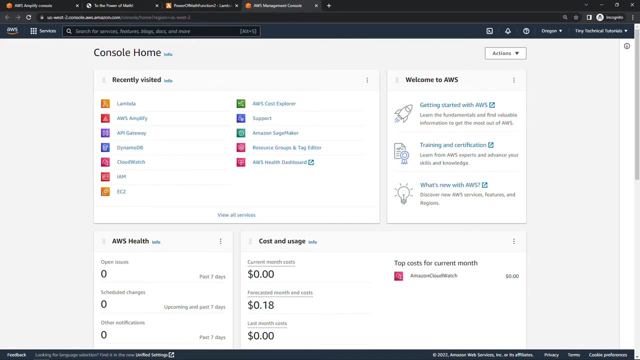 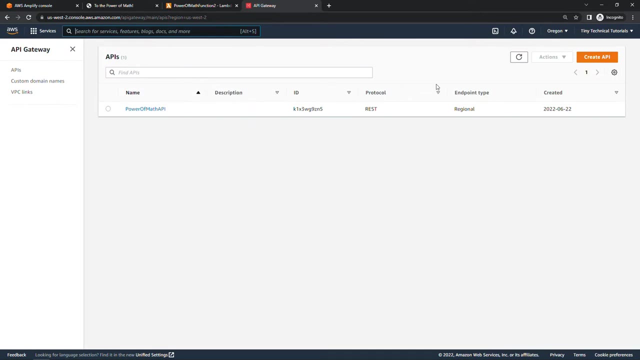 and do that All right back here in the browser. I'm also going to open a new tab for this, just so we can keep all the services up and visible easily. And for this one, we're going to navigate to API gateway. Once again, this is my original API. let's create a new one by clicking on the. 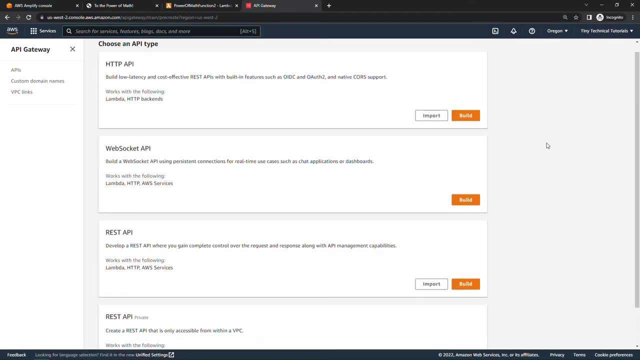 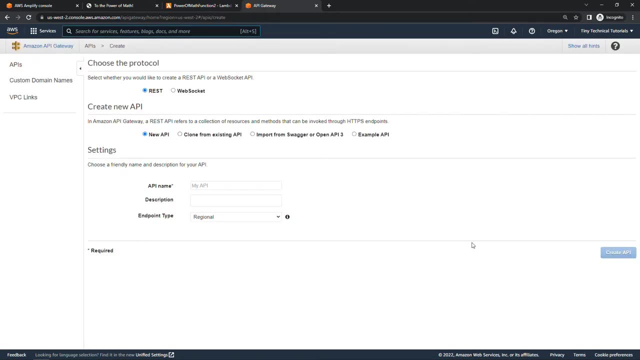 create API button up here. For this we're going to be using REST API, So here on this section, click on the build button. You can leave these first two options as they are. So this will be REST and a new API, And then we need to give it a name, So mine will be Power of Math, API 2.. 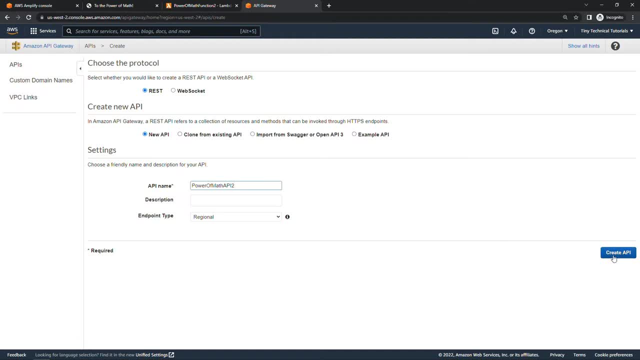 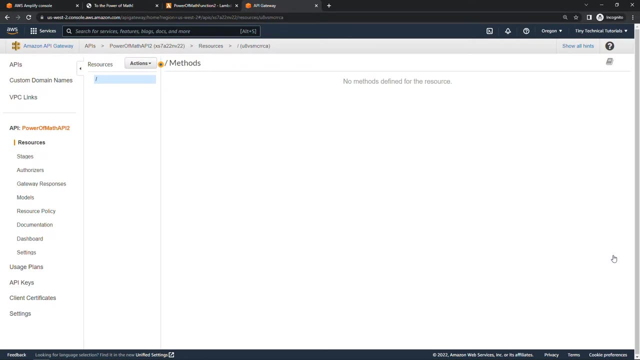 You can leave everything else the same and then create API. Okay, so we have sort of an empty API right now. There's no methods that somebody would call, So let's do that next Over here on the left, make sure you have resources selected And then here. 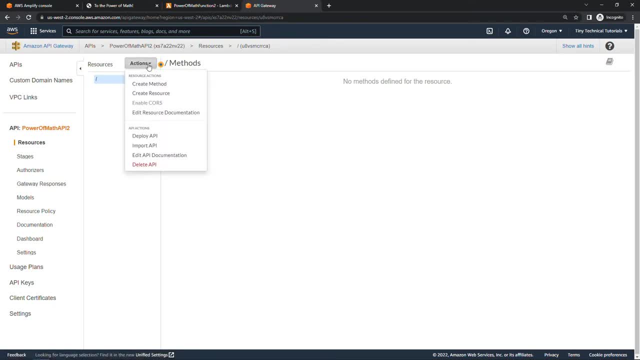 the backslash selected And then on the actions menu, create method. The type of method will be a post. So remember the user is sending in some data, those two numbers, And then click the little check mark right here For integration type. we're going to use a lambda function And then 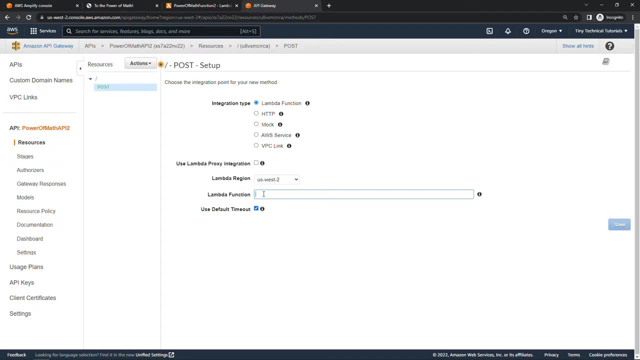 the lambda function name itself. you'll need to start typing in here, But it should be Power of Math And in this case, function two for me. click on save And okay. here we're giving API gateway permission to invoke this lambda function. 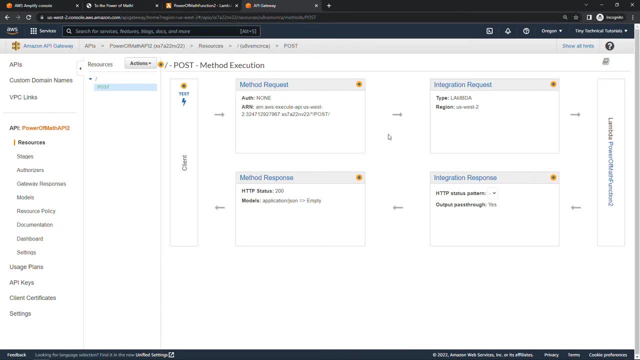 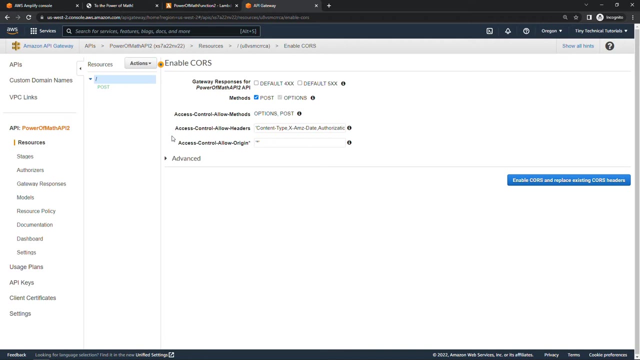 Now one other thing we need to do is enable cores, or cross origin resource sharing. So come over here and make sure you've got post selected And then, on the actions menu, enable cores, And basically what this does is allows a web application running in one origin or domain. 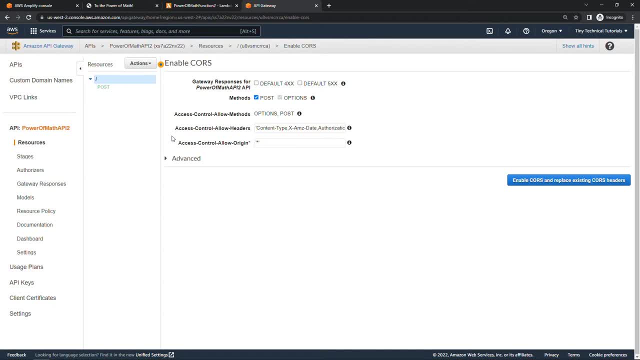 to be able to access resources on a different origin or domain. So because our web application is running on one domain and amplify our lambda function is going to be running in another. we need to be able to work across those domains or origins. That's why 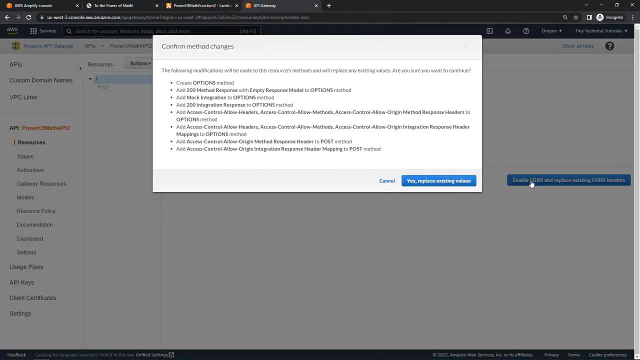 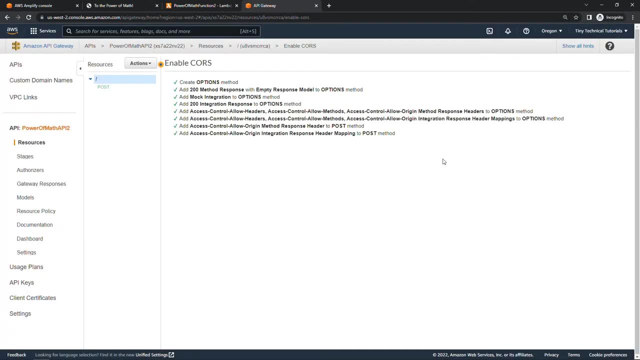 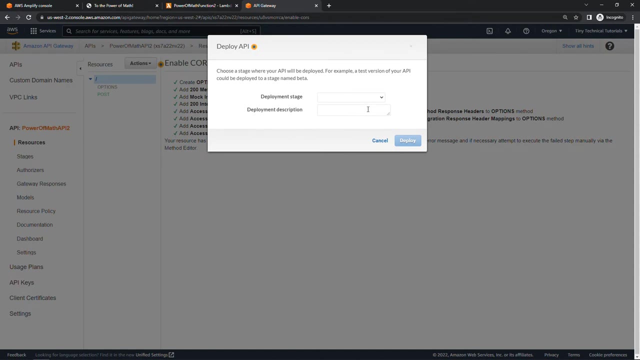 we're doing this. You can just click on enable cores And yes. And now let's deploy the API so we can test it out. So up here again on the actions menu, let's deploy API. We'll need to set up a new stage here. You might have different stages for dev. 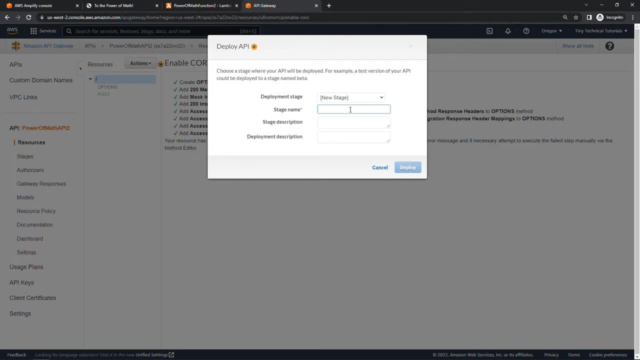 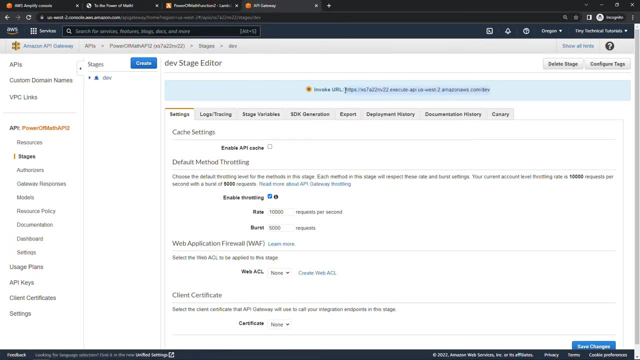 test, production and so on. This one we'll call dev and deploy, And then you'll need to copy this URL right here, the invoke URL, And we'll need that later. So just pull up a notepad or wherever you want to keep this. I'll do that myself now, And just so I can. 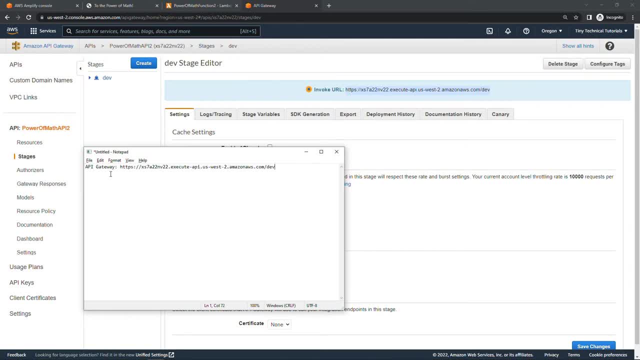 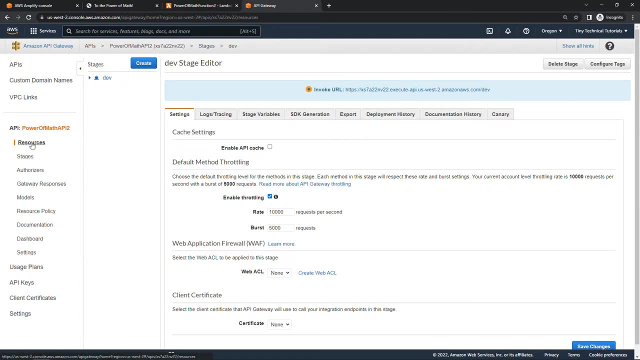 keep things straight, this will be the API gateway URL And I'll just save that for later. All right, now let's go validate this. So over on the left, come in to the API gateway And I'm going to resources. Click on post And here you'll kind of see a flow of how this works. So we have the. 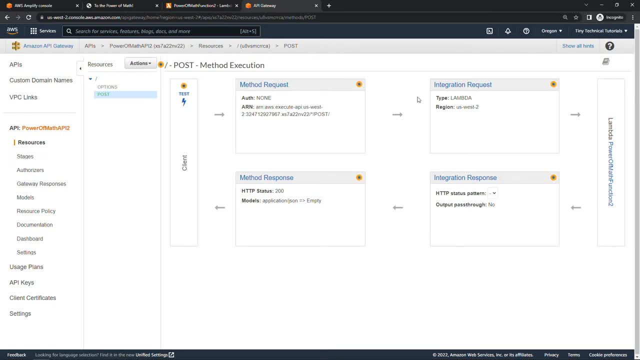 method request, the integration request to Lambda. Lambda is going to work its magic And then we're eventually going to get this response back to the client, to the browser. So we want to test that this is working. To do that, click on the blue lightning bolt here And this will. 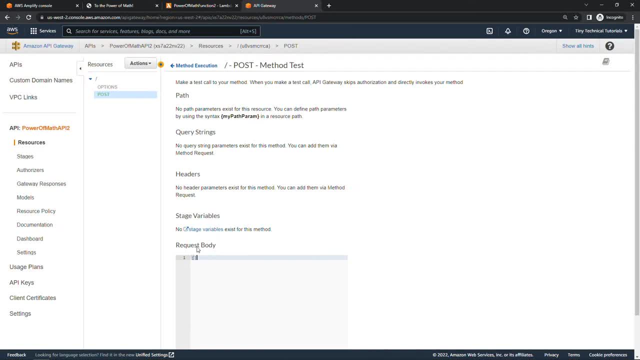 let us send in whatever test data we want. So we'll just keep it simple. It's the same format. We'll use this particular page. This is what we're going to твор and load, so in this process, we will be able to develop this loan test And then we have all of our block and plan to clickvolve way to get even bigger resources. I'll also have� 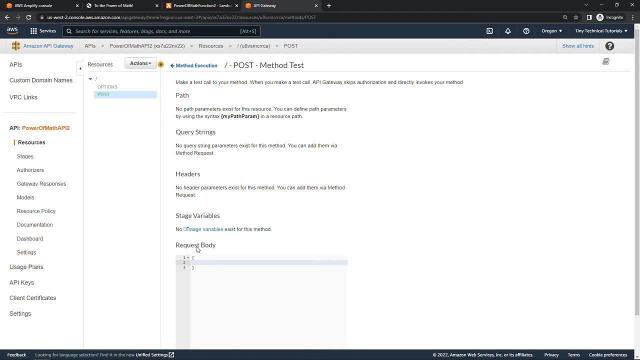 We'll just keep it simple. It's the same format we used to test lambda actually. so we'll have base and let's say two comma, and then the exponent number, And maybe we want to try with, say, four. 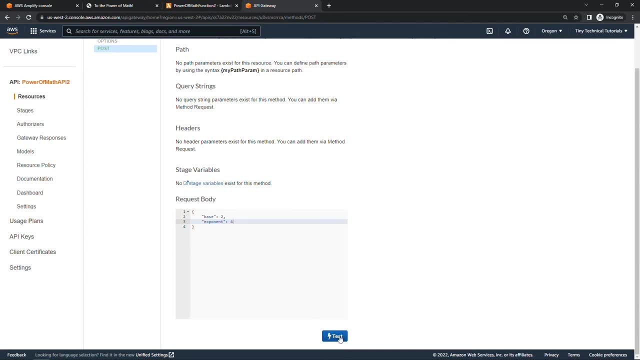 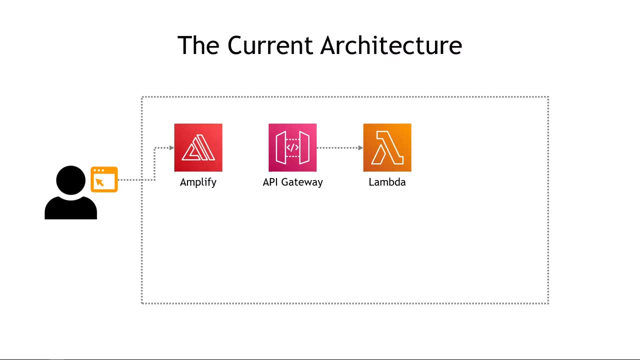 Okay, now let's test. And here's the result: 16, everything worked. yay Progress. Now we can trigger our math function in lambda with an API call. We still haven't hooked that up to our indexhtml page in Amplify yet, but don't worry, we'll get there. 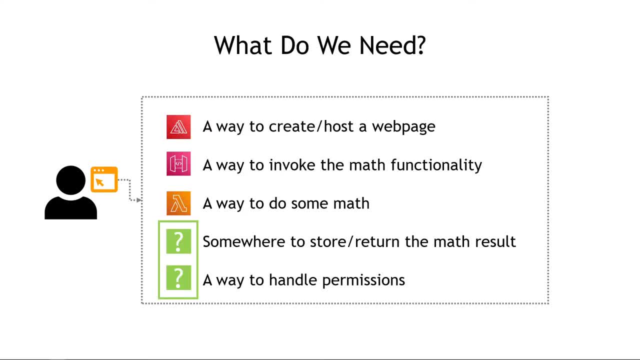 Next, though, let's see how to incorporate a database into all of this. We want to persist or store that math result somewhere, and we obviously need to return it to the user as well. Now, maybe I should rephrase that We don't actually have to store the results anywhere. 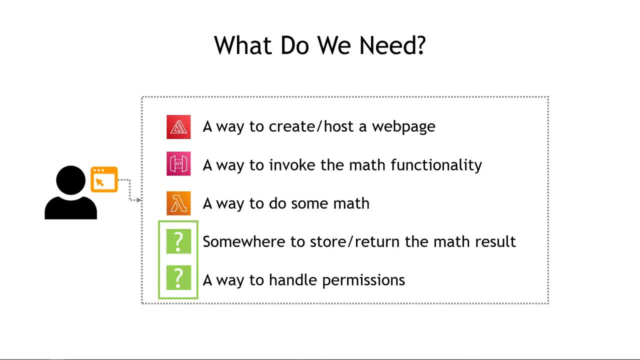 We could just return them, but most real-world apps these days have databases, so I'll walk you through how to set this up. As we do that, we're also going to need to handle permissions between the different parts of the application, Starting with the database. for our purposes, 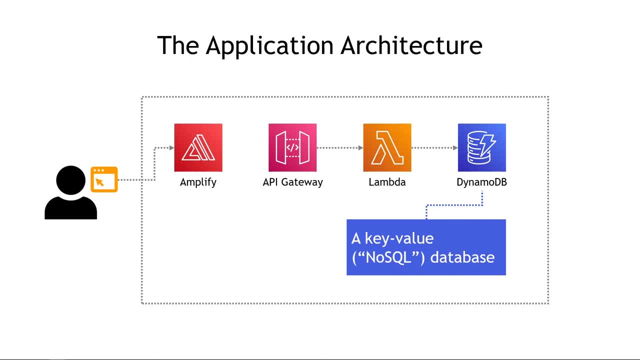 we're going to be using DynamoDB. This is a key value or NoSQL database and it's generally going to be lighter weight than something like a relational database where you have to go set up your schema, your relationships and so on ahead of time. 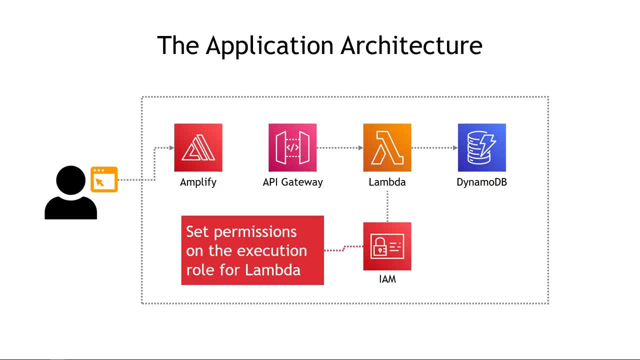 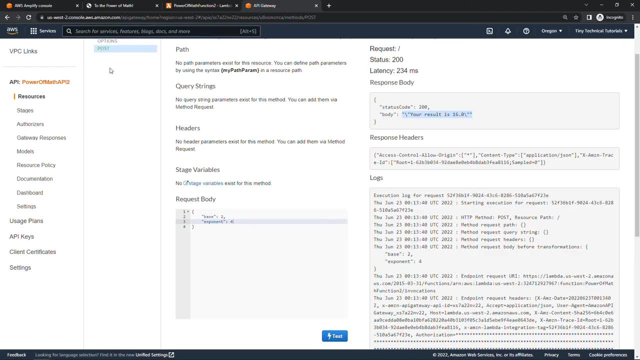 And then I mentioned a second ago that we have to deal with permissions as well. Specifically, we're going to need to give our lambda function permission to write to the database, so let's go work on this next. All right, once again, I'm going to open a new tab. 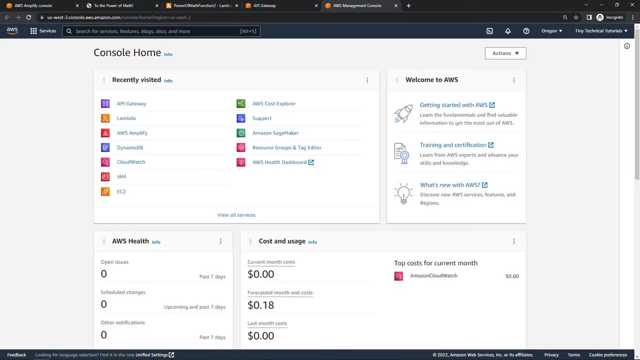 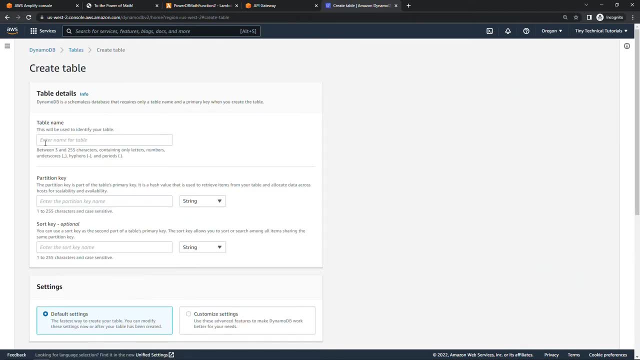 so we can keep this one dedicated to DynamoDB, And here we want to create table. For table name I'll do Power of Math Database. 2. For partition key, we'll say ID. You can leave everything else the same and create table. 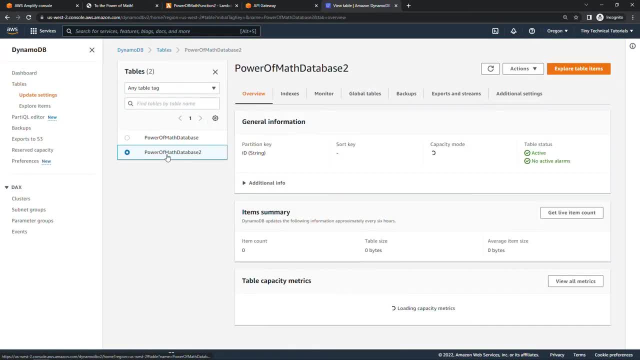 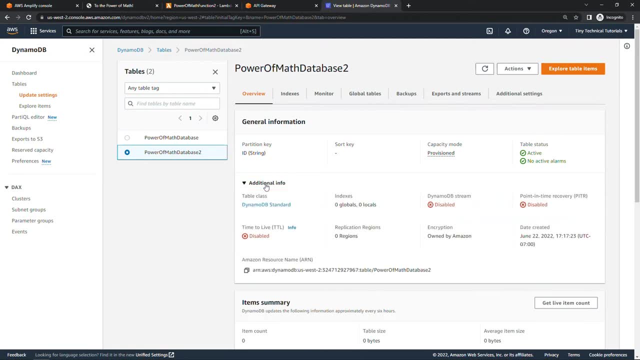 Okay, now we do need to save the Amazon resource name or the ARN for this. So if you click into that table and, under General Information and Additional Info, grab this ARN right here and then just paste that into the same notepad. 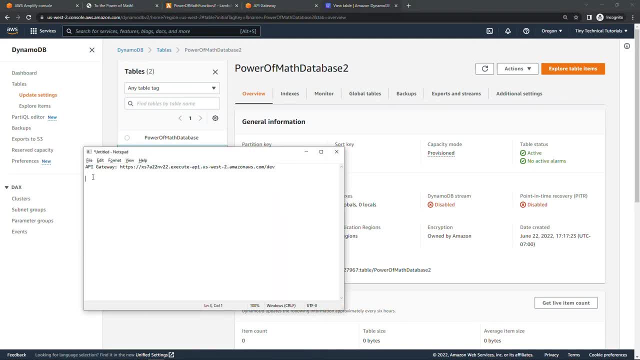 or whatever you're using to store your links. So this is my ARN for the database and we'll come back and get that later. All right now, moving on to that permissions discussion. this has to do with our lambda function: having permissions. 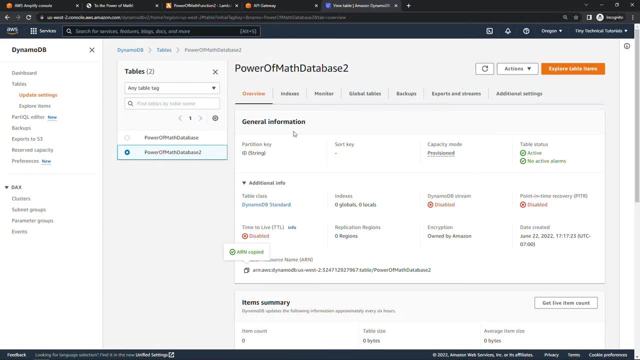 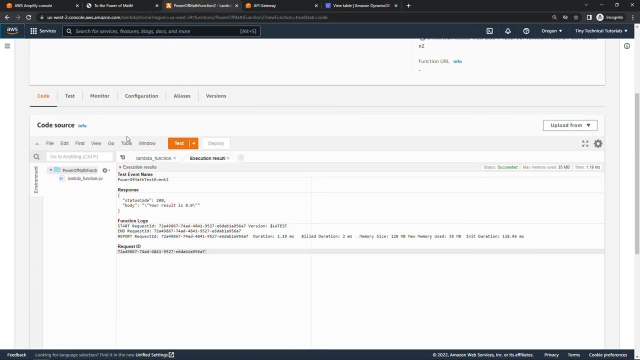 to write to this table. So we'll come back to our lambda function here, the Power of Math, function 2, or if you've closed that tab, just navigate back to lambda and find this function And you'll want to go to the Configuration tab here. 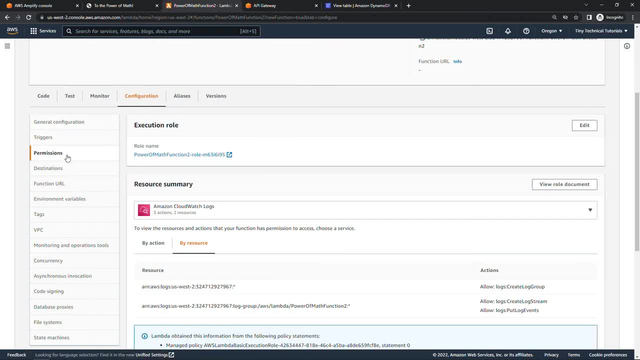 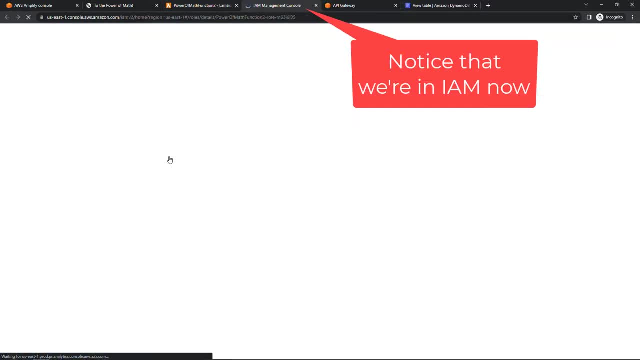 and then, if it's not already selected, go to Permissions, and then you'll want to click on this role name here, the Execution role. This should open up in a new tab and we basically need to add some additional permissions to what this role has already. 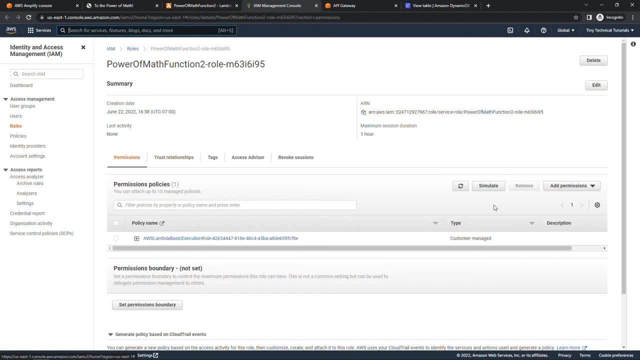 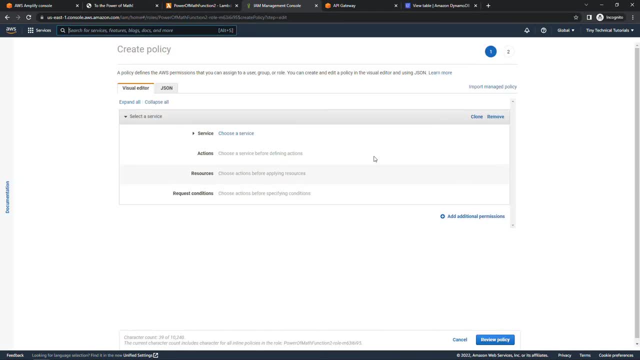 Permissions related to DynamoDB. To do that, come over here to the right, Add Permissions and Create Inline Policy. And then I personally find it easier just to work with the JSON code. so click on the JSON tab here and let me go grab the code that we need to put in here. 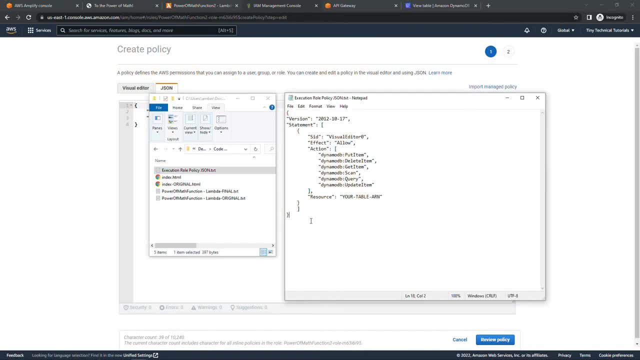 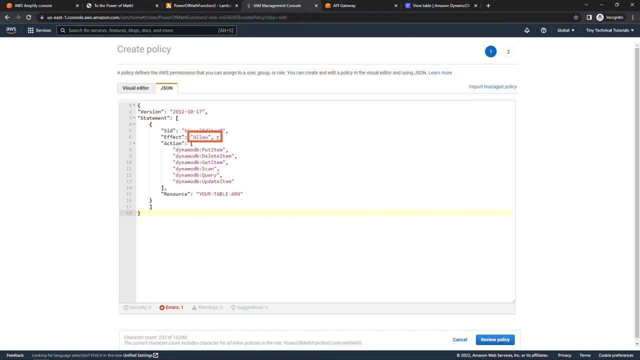 This again will be linked in the description if you want to grab it. But I'll just copy all of this and replace what I have here, And this is just basically saying allow, and then I'll just copy all of these different actions in DynamoDB. 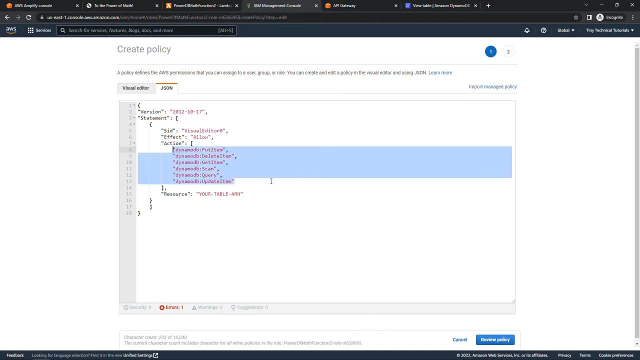 So the lambda function's gonna have permissions to do all of these things on our DynamoDB table, But, very importantly, you need to update this right here to that table- ARN that you copied just a minute ago, So let me grab mine. It's this one right here, starting with ARN. 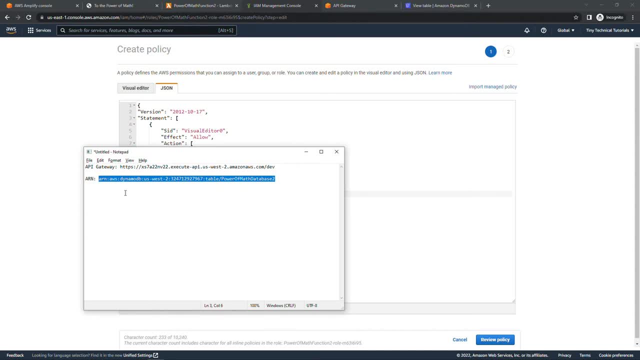 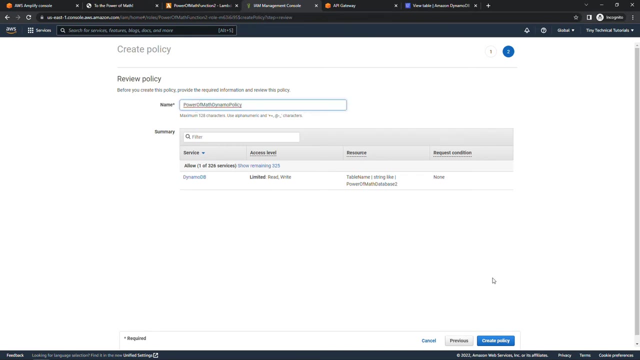 the lowercase ARN colon, AWS colon. So I'll copy that, put that right here. Then we'll Review Policy, We'll give it a name: Power of Math, Dynamo Policy And finally Create Policy down here on the lower right. 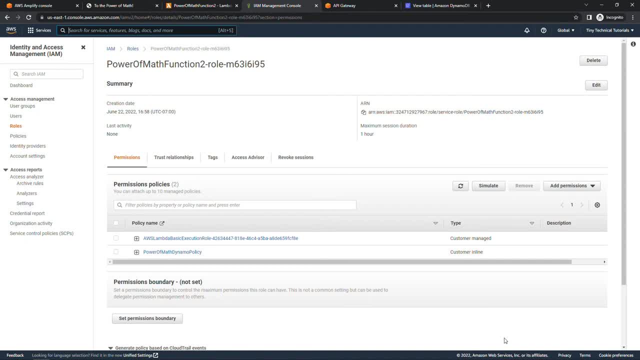 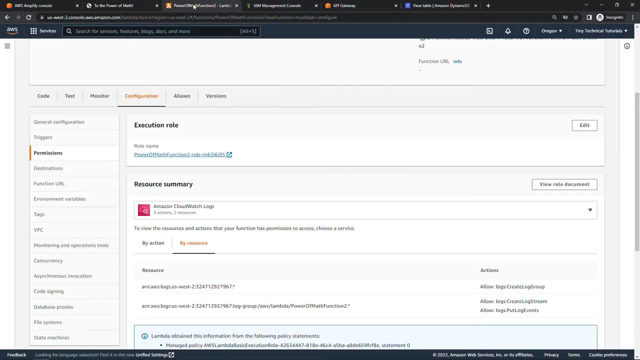 Okay, so that was the permissions thing that we needed to get through. Now we can update the lambda function to actually go right to the database. It wasn't doing that before, So let's come back to the lambda function here and code, And if you still have your execution results up, 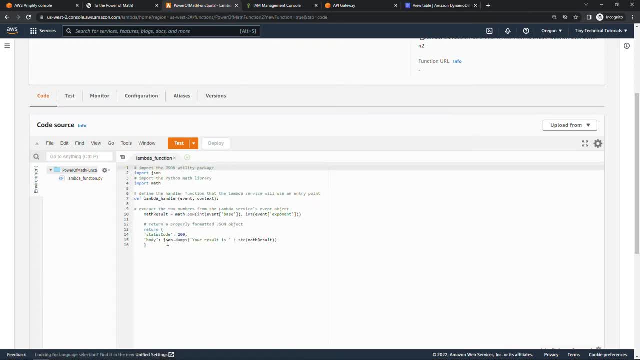 you can just close those. We want the functionpy here, your Python code, And for this one I also have some code completed that I'll just paste in. Let me grab that. This one's going to be Power of Math Function Lambda Final. 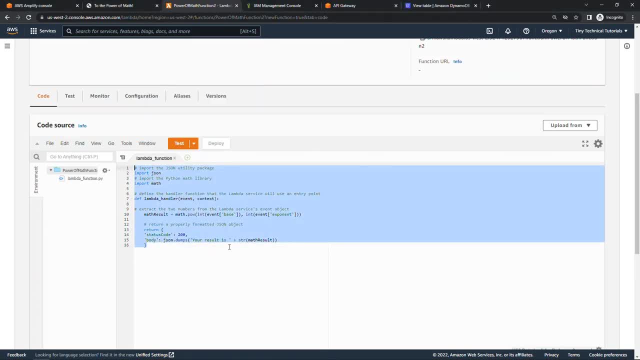 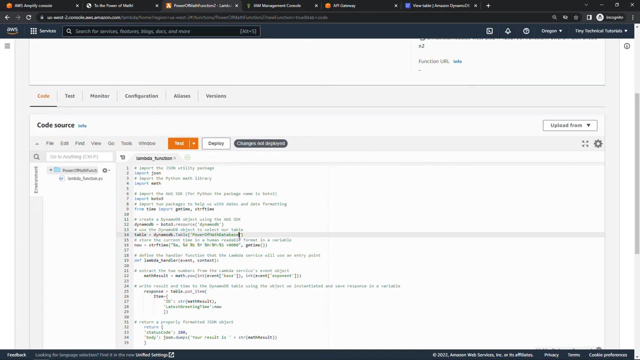 So I'll grab all of this, paste it in here replacing everything. Now I do need to make an update to my table name, since I'm using a 2 at the end of mine, So I'll just walk you through what's new here. 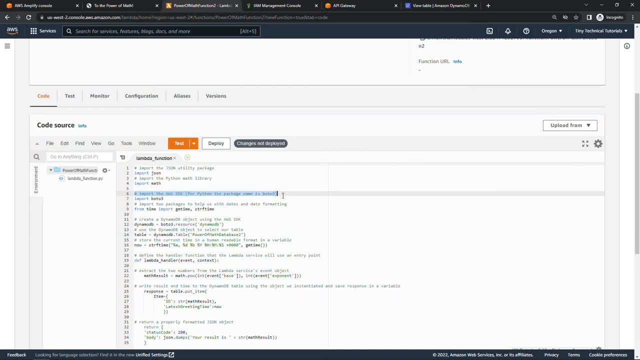 So we have two new imports up here, one for the AWS SDK Software Development Kit And, because we're using Python, this one's called Boto3.. And then we've got some packages here that help us with date and date formatting. 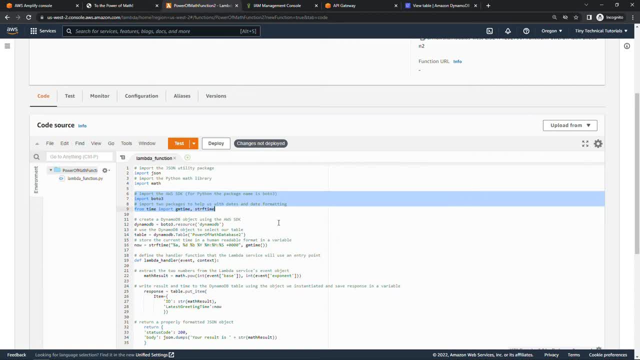 So when we go to insert our math result into the DynamoDB table, we're also going to insert the current time, And that's what we're doing right here is working with the DynamoDB table. So we're getting our Boto3 resource for DynamoDB, grabbing the table. 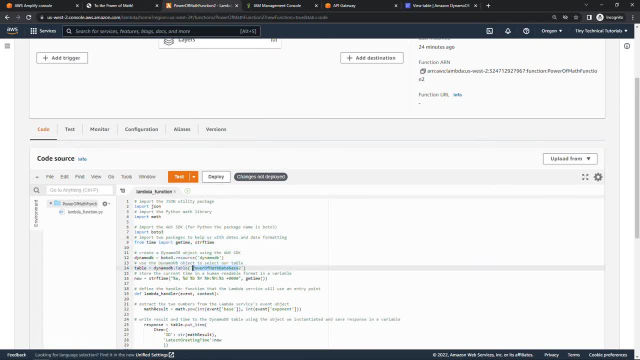 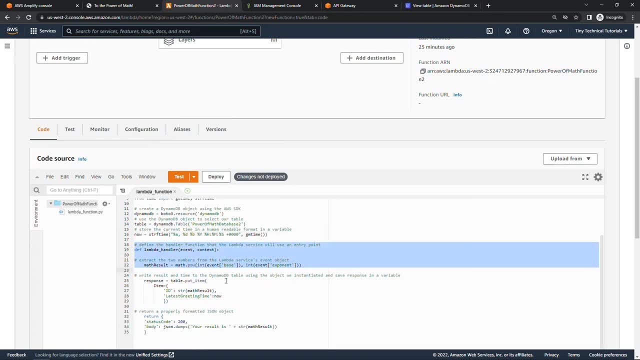 So in my case this was Power of Math, Database 2.. And then getting the current time. The rest of this is the same as what we had before, but the code that actually inserts into the table is with this tableput item, And then we're inserting the math result along with the time. 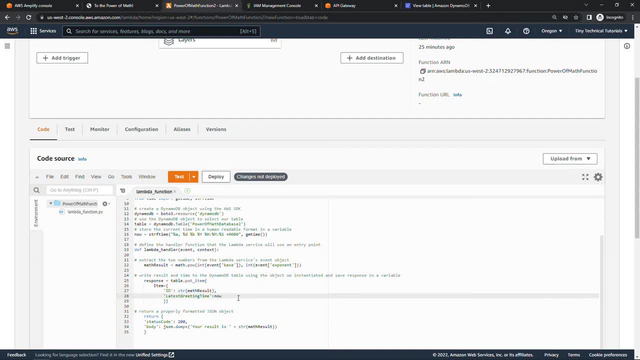 So just a few minor updates from what we had before. All right, so paste in that updated code, Make sure you save with a Control-S. Very importantly, make sure you deploy. This pushes out your changes And then let's test. 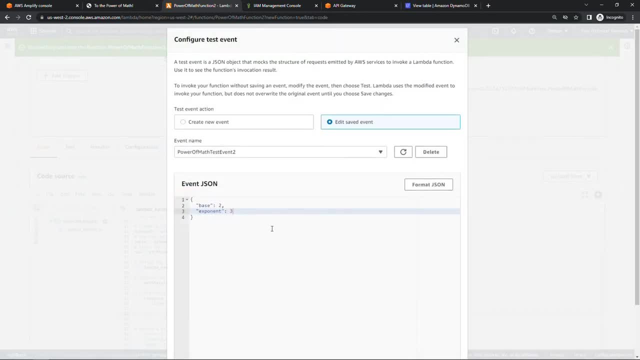 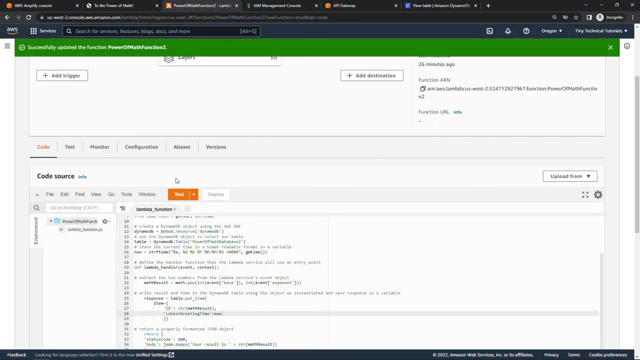 So we should still have the same test case back here, or test event: A base number of 2, exponent of 3.. You can change that if you want, But let's just hit Test and see if we get the correct result. 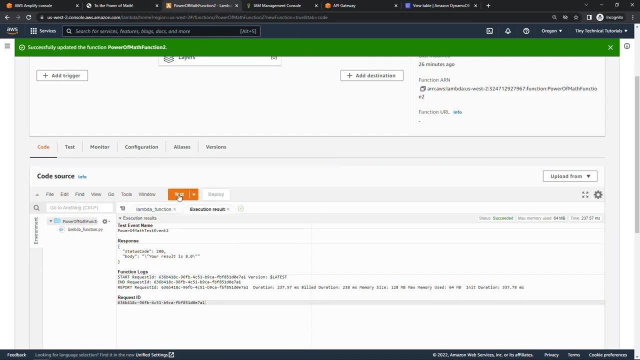 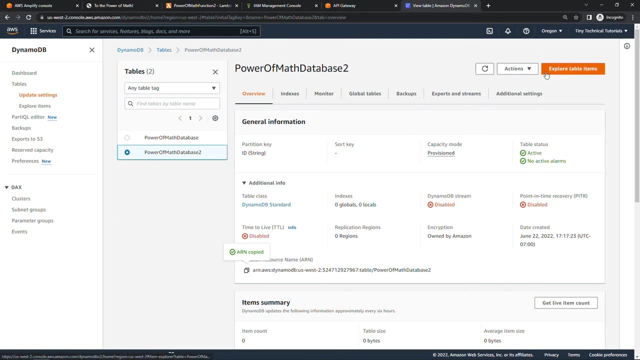 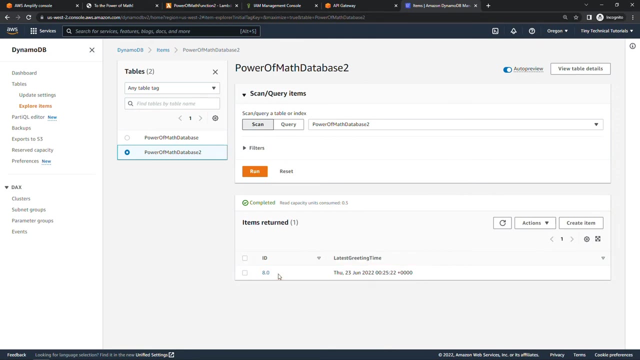 Yay, your result is still 8.. But this time, if we go look at our DynamoDB table back here and we come into Explore Table Items, this will show you what's been stored there. We have a result now, So this is the one that just came through from us running that test. 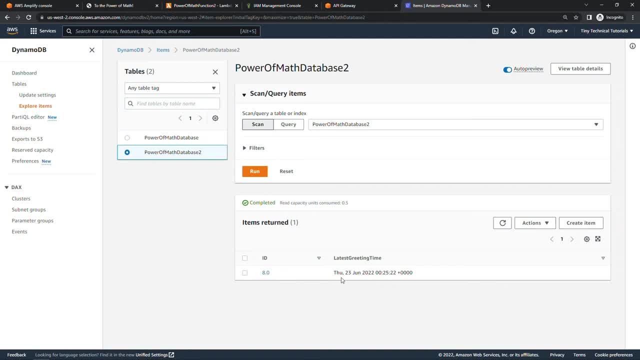 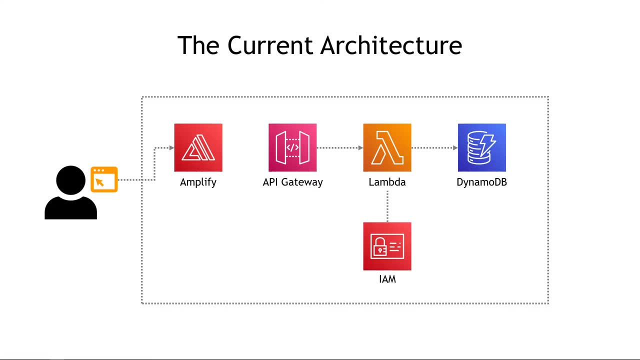 So this was the math result here: 8.. And then the time that that happened. All right, things are looking good. We're writing things to the DynamoDB table. We've got the proper permissions on the Lambda function. We're super, super close. 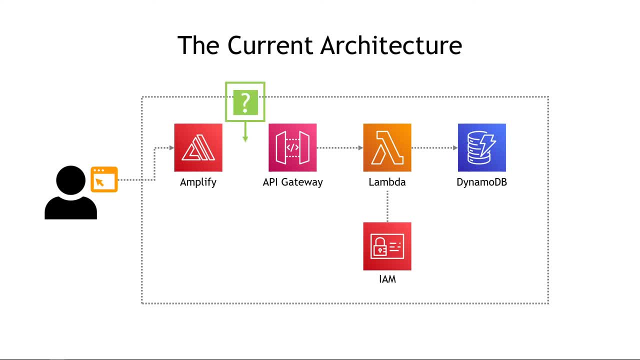 But you might have noticed that we're missing a connector here, And I didn't just mess up the diagram. We actually are missing a connector here between Amplify and API Gateway. We've built out all this goodness over on the right, But currently from our indexhtml page there is no way to get to it. 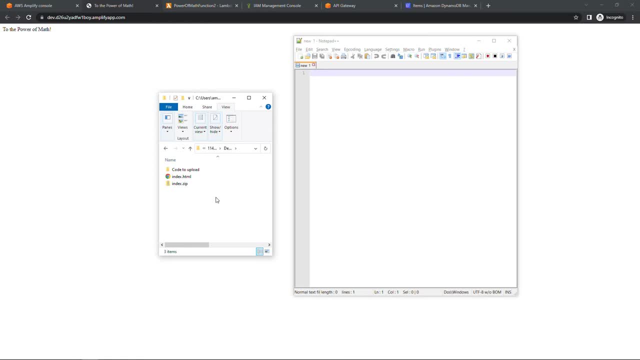 So let's work on this final piece. For this part, we're going to need to update the indexhtml page, So go ahead and open that up. I'll open it in Notepad++ And remember: this code is what's giving us this over here. 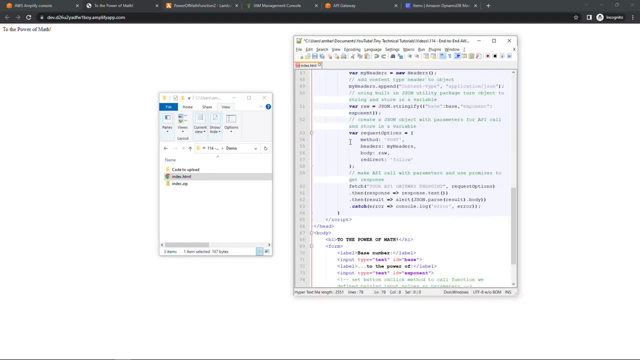 I'm going to paste in the final code here, So definitely not something you want to type. If you're grabbing it from the description below, it'll just be the indexhtml. The original was just a simple one. that's giving us that. 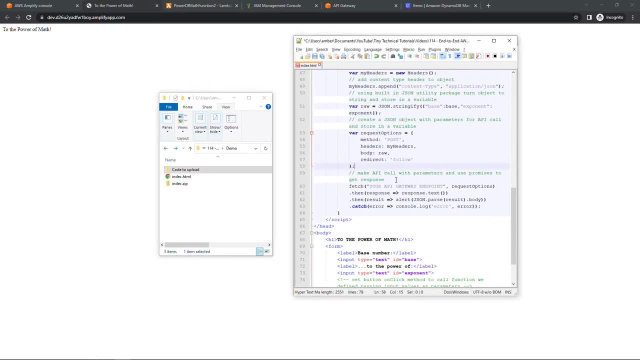 So make sure you're grabbing that one there And I'll walk you through the code here. Let me collapse this to make it a little bit easier. So first I've just done a little bit of a styling update- Definitely personal preference here. 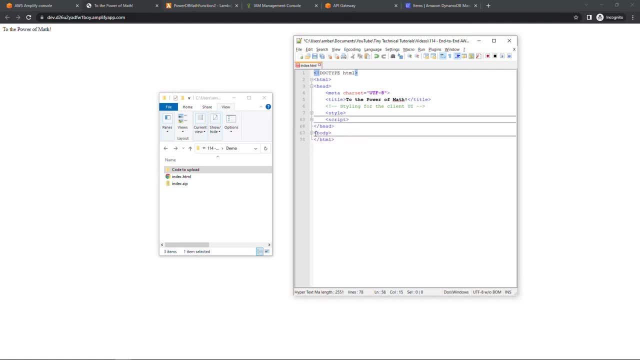 Feel free to update any of this CSS code And then down here under Body, we have an H1 tag here to the power of math, So that'll be our heading And then the form. So this is where the user is going to input their two numbers. 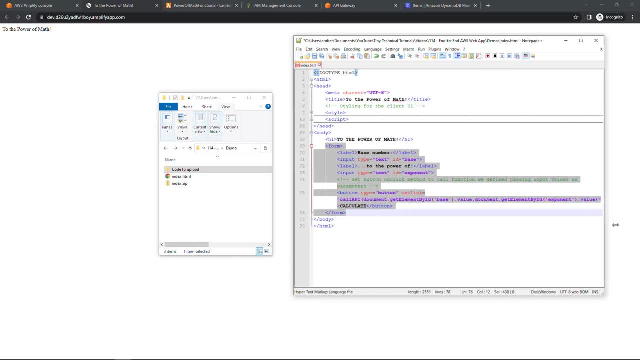 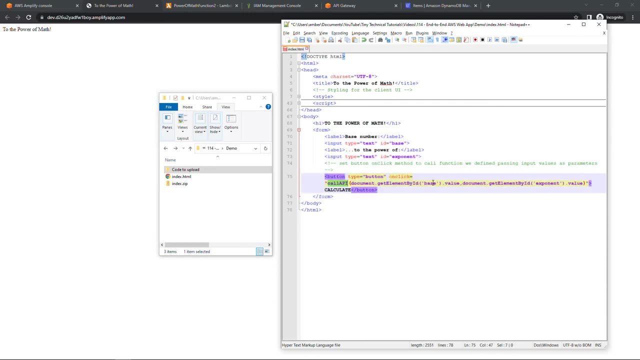 And then we have a Calculate button here as well. Increase the size a little bit. But the magic really happens here with this call API. We're passing in the base and the exponent, those two numbers, And call API is defined right up here in the script tag. 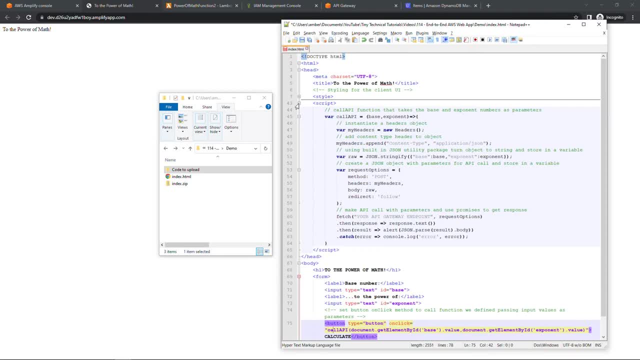 And this is what's hooking us up to our API gateway endpoint. But, very important though, you need to update that with your URL, So let me go grab that for mine here. It should end in dev. if you created a dev stage, like I did, 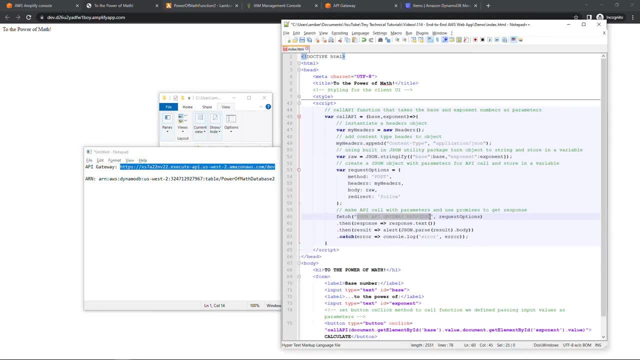 So I'll grab that, Update this here. But this is basically the code that is going to pass your base and exponent to the API gateway endpoint And ultimately we're going to get this alert back with the result of that calculation, The alert being just the pop-up that we saw there in the browser. 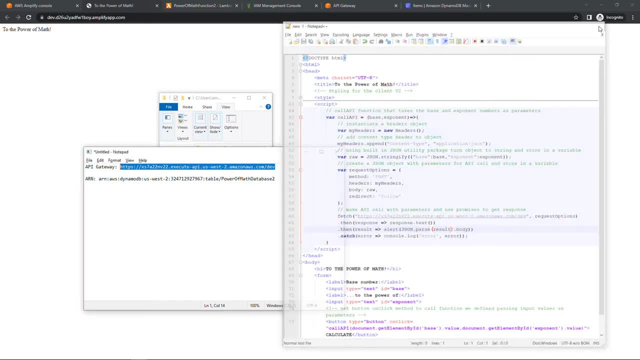 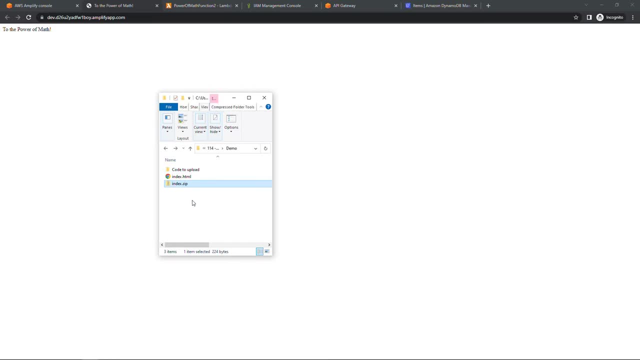 All right, let's save this. I'll close out of that, Close out of that. And then we need to make a zip file out of this again. So I'm going to save this. I'm going to delete our original zip file. 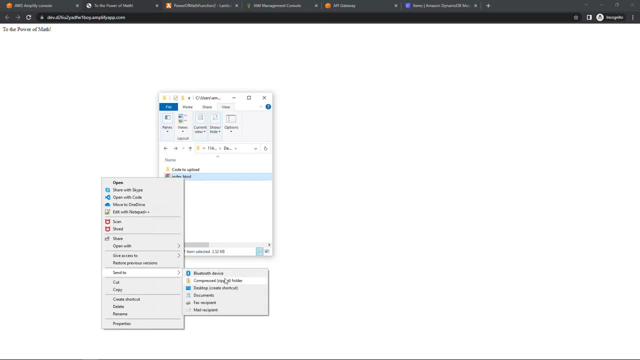 And then this is the updated indexhtml We'll send to compressed folder. So there's our new zip And then we're going to need to go redeploy it using Amplify. So I've got Amplify open in this first tab back here. 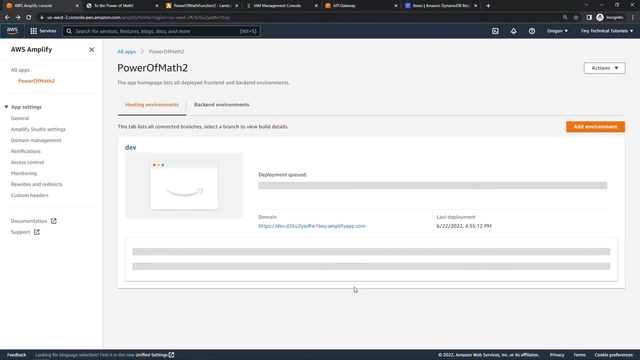 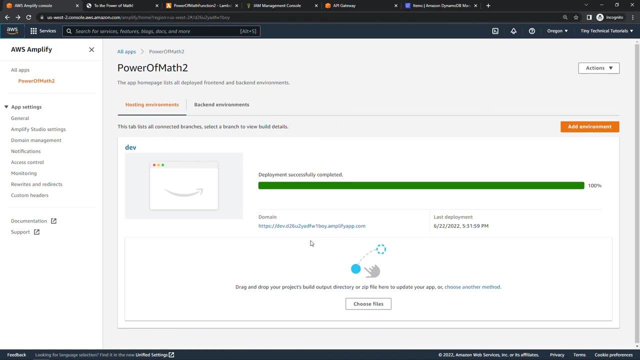 Just grab the zip file, Drag it over here And this will automatically redeploy. So deployment is queued And success. So it should be the same domain here. You can open it. You can open it again or just come back to the one that we had open from earlier. 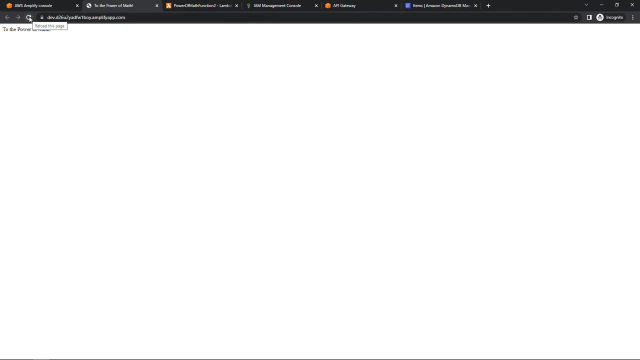 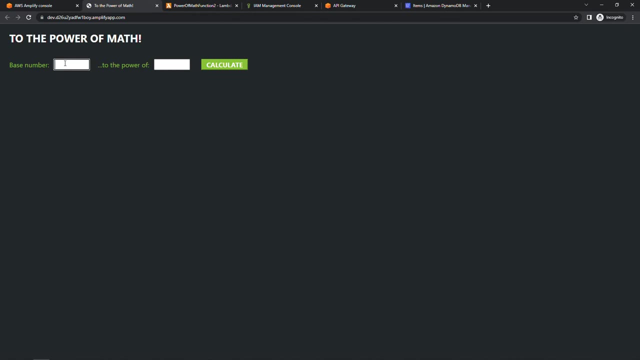 And I'll do a refresh. So this is our original one. Let's see what we have now And ta-da, Some style. All right, so let's walk through what's happening here. We're going to enter our numbers. Let's just say 2 to the power of 8 for something different. 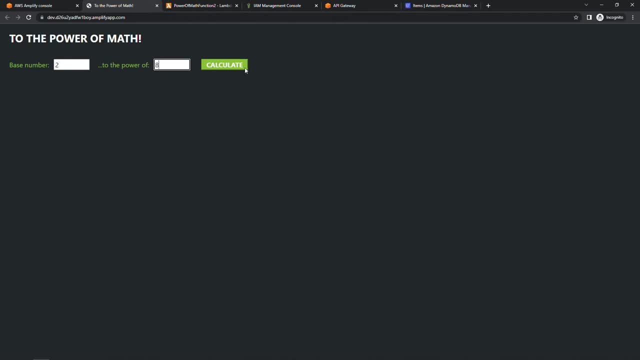 When we click this Calculate button, that script here on our HTML page is going to call API Gateway. That's then going to trigger the Lambda function Which does the calculation. That gets written to the database And then we're going to get a message returned to us in the browser through API Gateway. 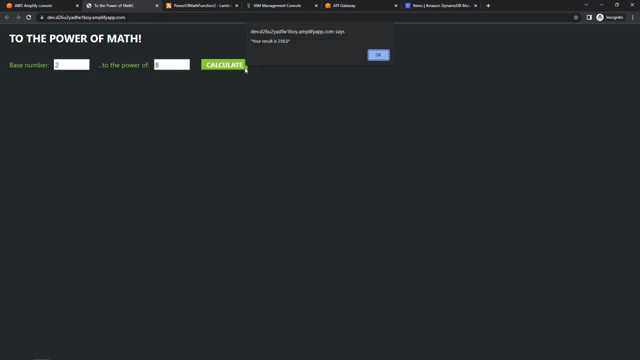 So here we go, Calculate, And the result is 256.. All right, that's our completed application. Nicely done. I hope you were able to follow along and have a working application yourself. This is a link that you should be able to share with your friends if you want. 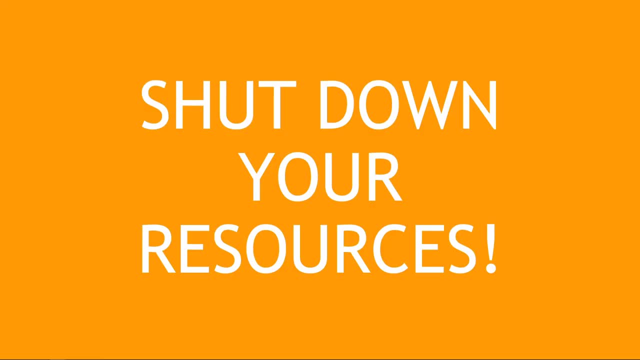 All right now, before you go run off, a very important reminder. If you've been following along, let's go delete everything that we spun up in the video. Everything should be in the free tier, but just in case you don't want any surprise. 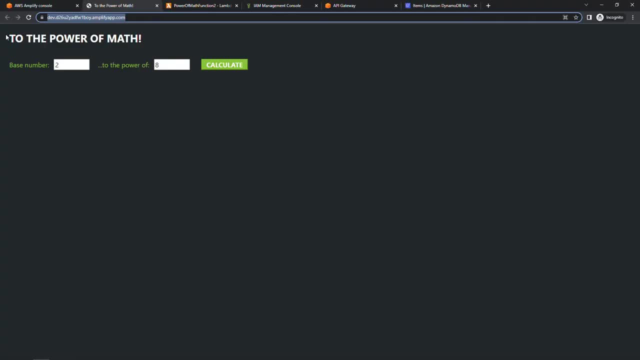 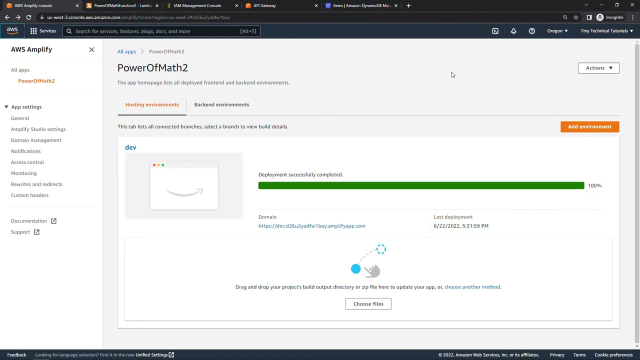 bills at the end of the month. So I'll walk you through how to delete things. I'll just close out of this tab where the app was And then coming into Amplify your app. you'll want to come up to Actions on the top right. 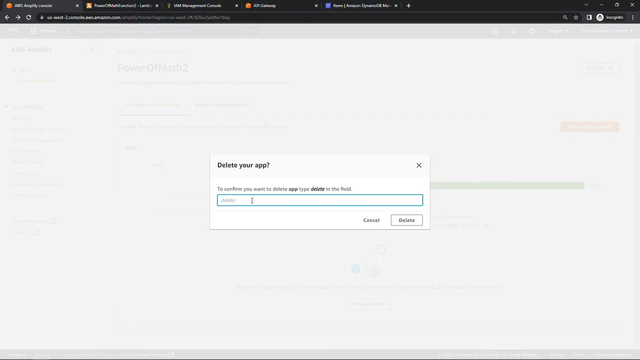 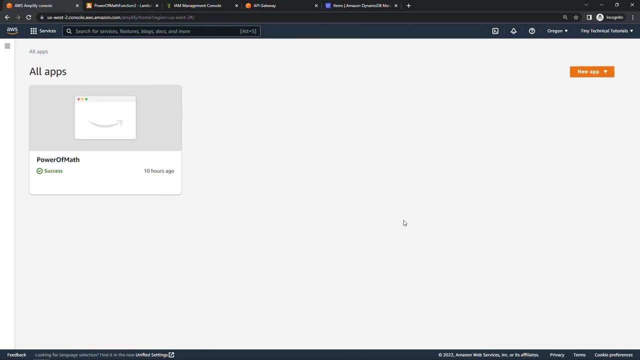 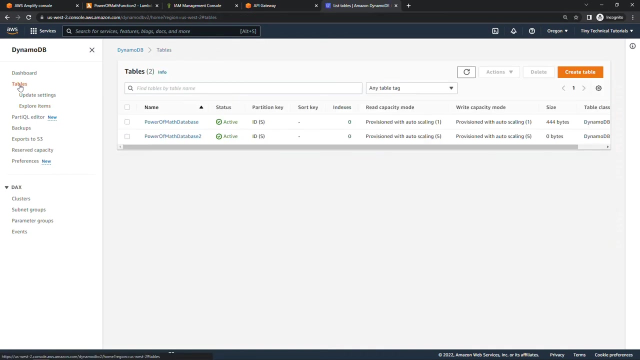 here and Delete App. You'll need to confirm. This is my original one that I will keep for now. Next come over to DynamoDB And I'll click on Tables over here just to make sure I'm getting the right one. This was Power of Math, Database 2.. 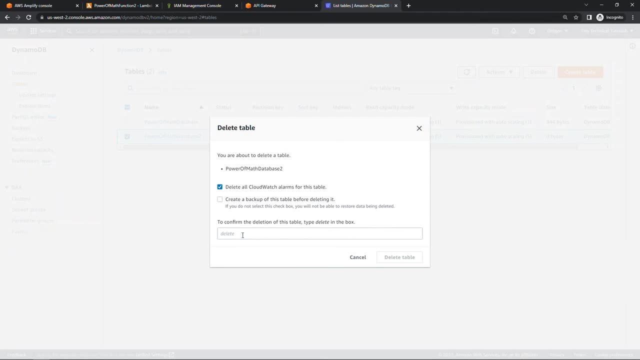 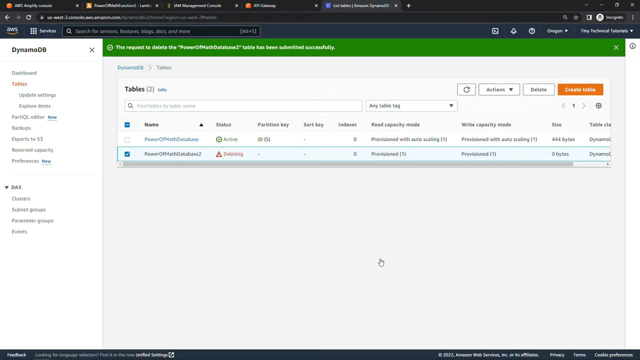 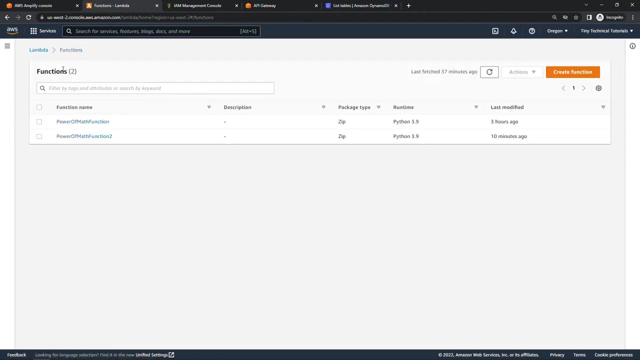 And up here you can say Delete- This also has confirmation required- And Delete. Next you can go delete your Lambda function. So back here, Power of Math, Function 2. Or if you're at your Functions top level, Just select that. 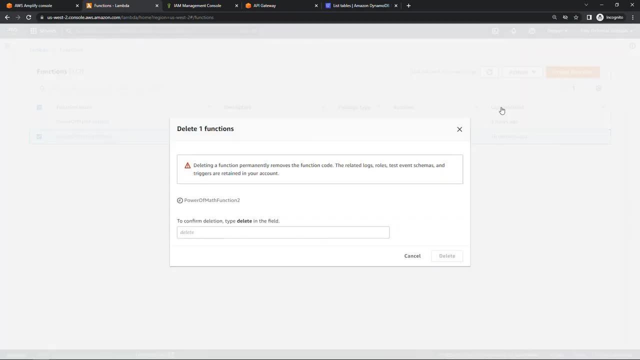 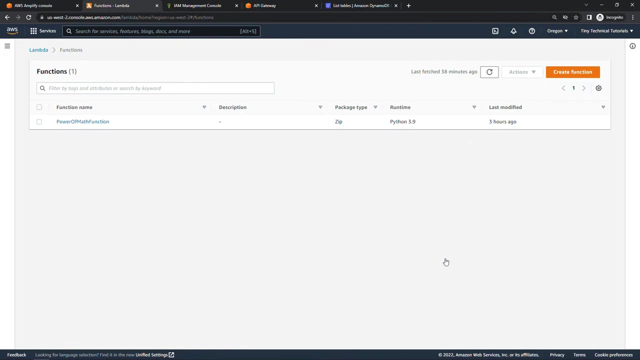 And Actions and Delete, Delete And OK Or Close, And then, lastly, API Gateway. Come here back up to APIs, And I'll delete this one as well. So up under Actions and Delete And with that, one final thing to do, if you haven't already. 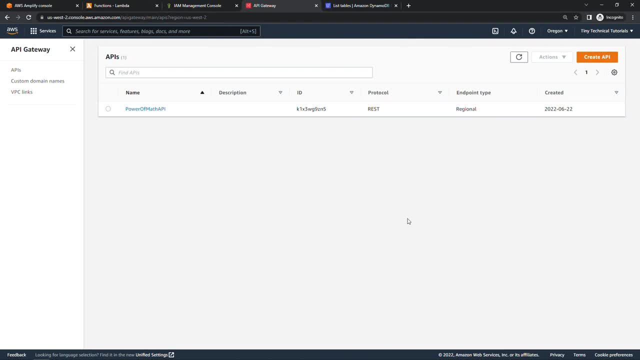 Go, hit that Like button And also consider subscribing for more content like this. Thank you so much for watching. I hope you found this helpful.